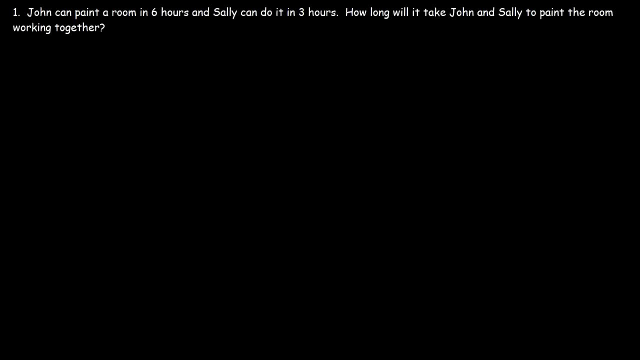 In this video, we're going to work on some work-in-time problems And there is a simple formula that you could use that can help you to get the answer quickly, And we're going to explore that today. So let's begin with this problem And, by the way, for each of 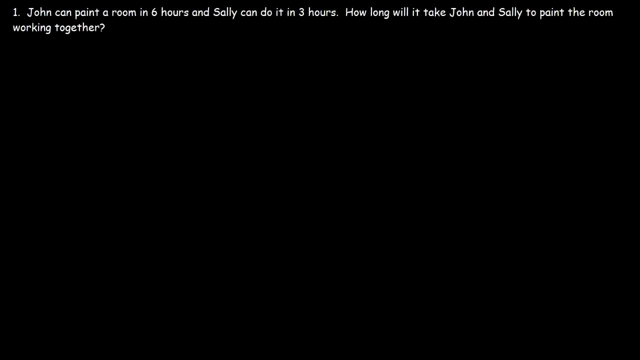 these problems. I recommend that you pause the video and, you know, give it a shot. Try it out first to see if you can get the answer. So let's go ahead and begin Number one. John can paint a room in six hours And Sally can do it in three hours. How long will it? 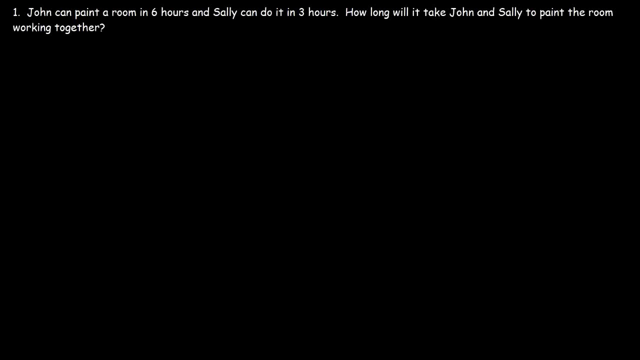 take John and Sally to paint the room working together. So how can we find the answer to this question? What do you think we need to do? What formula should we use? And there is a simple formula that can help you to get the answer. So we're going to say: 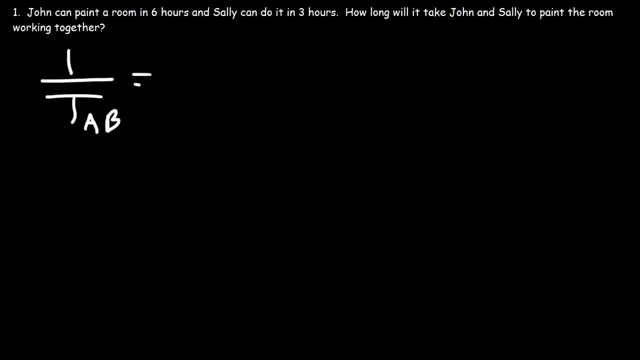 here it is: 1 over TAB is equal to 1 over TA plus 1 over TB. In this case, let's adjust the letters A and B to the first letters for John and Sally. So we're going to use J for John, S for Sally, So TJS would represent the time it takes for John and Sally to paint. 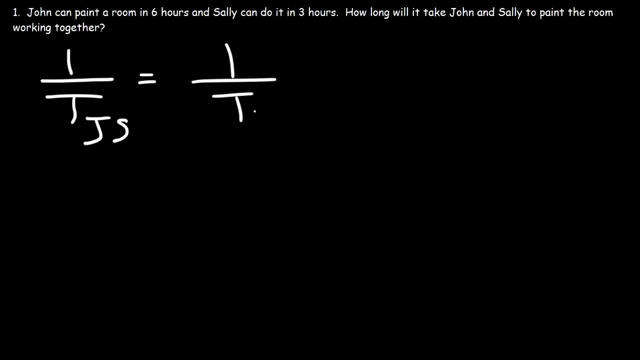 the room And let's change the number to 1 over TAB, because that is the number we're going to use, And let's say we decide the number of hours for John and Sally to complete the job. TJ is simply the time it takes to John to complete a task working alone, And 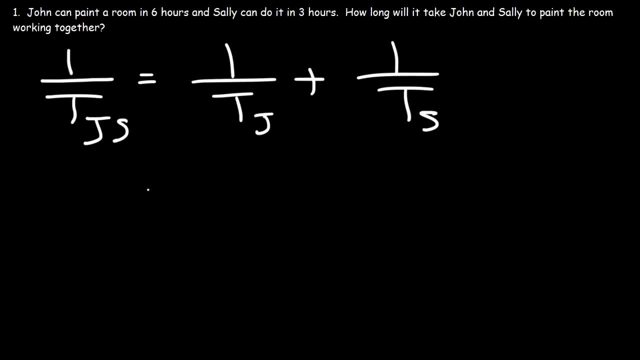 TS is the time it takes Sally to get the job done by herself. So what we're going to do now is replace TJ with 6, because John could do it in six hours, And let's replace TS with 3.. So at this point, if you don't want to write this whole variable, you can just replace. 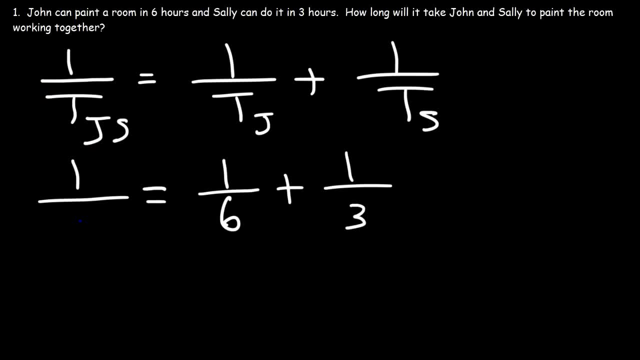 with x, because that's the missing variable that we're looking for. So let's just call it x. So how can we calculate the value of x at this point? What do we need to do? So at this point, it's basically algebra. 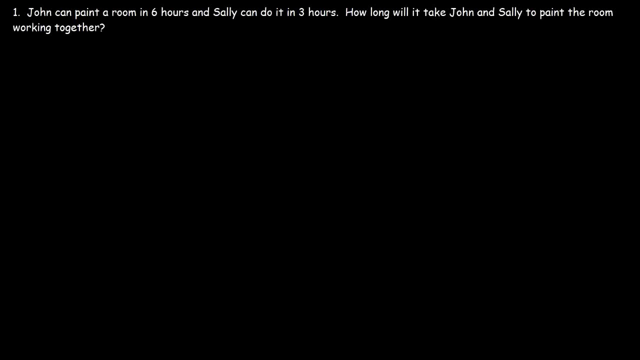 take John and Sally to paint the room working together. So how can we find the answer to this question? What do you think we need to do? What formula should we use? And there is a simple formula that can help you to get the answer. So we're going to say: 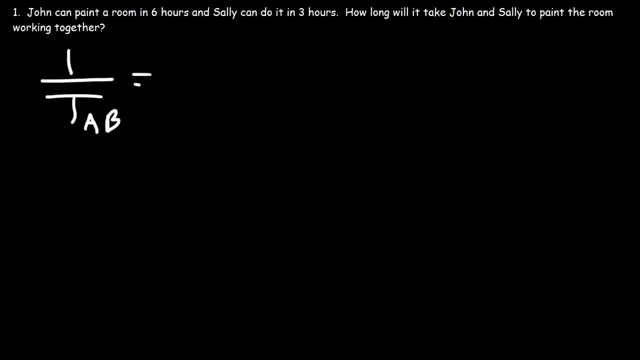 here it is: 1 over TAB is equal to 1 over TA plus 1 over TB. In this case, let's adjust the letters A and B to the first letters for John and Sally. So we're going to use J for John, S for Sally, So TJS would represent the time it takes for John and Sally to paint. 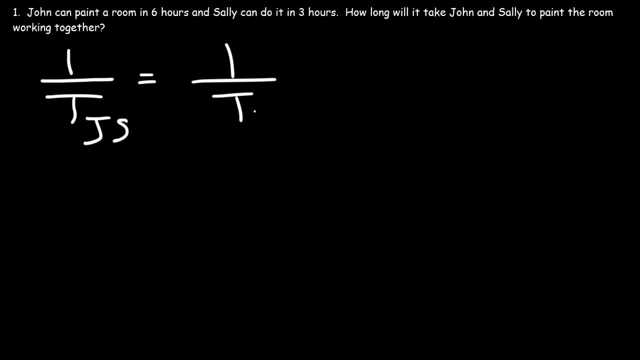 the room and to complete the job. TJ is simply the time it takes to John to complete the task working alone, And TS is the time it takes Sally to get the job done by herself. So what we're going to do now is replace TJ with 6, because John can do in six hours And 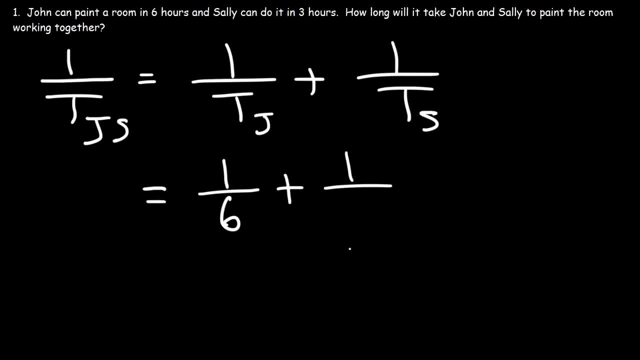 let's replace TS with 3.. So at this point, if you don't want to write this whole variable, you can just replace with x, because that's the missing variable that we're looking for. So let's just call it x. So how can we calculate the value of x at this point? 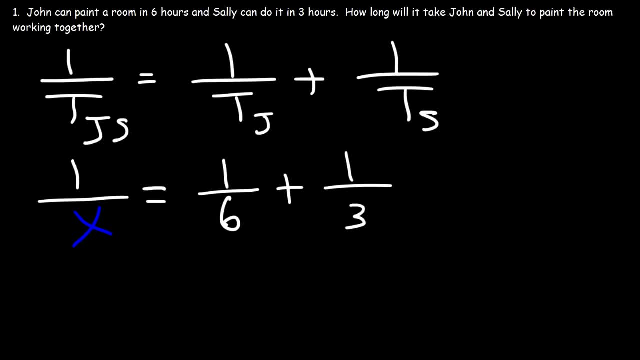 What do we need to do So at this point? it's basically algebra. You need to do some math here. Now, for those of you who prefer to get the answer just with a calculator, I'm going to show you how you can do that as well. 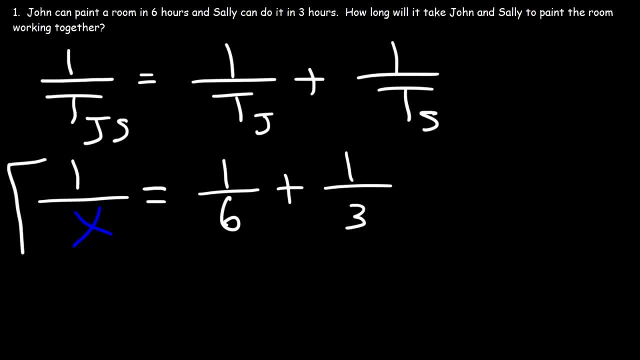 But for those of you who want to show your work, here's what you need to do: You need to multiply both sides, or basically every fraction in this equation, by something that will get rid of all of the denominators of each fraction. 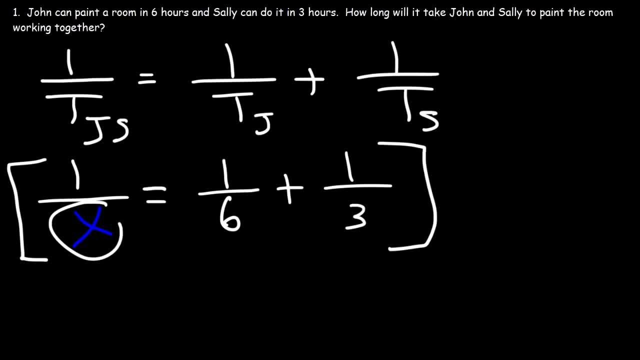 So what we need to do is find out the least common multiple of x, 6.. 6 and 3. And it's going to be 6x, So let's distribute 6x to everything inside the brackets. So let's multiply 1 over x by 6x. 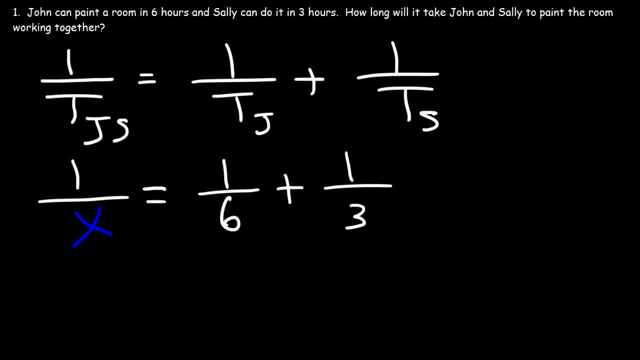 You need to do some math here. Now, for those of you who prefer to get the answer just with a calculator, I'm going to show you how you can do that as well, But for those of you who want to show your work, here's what you need to do. 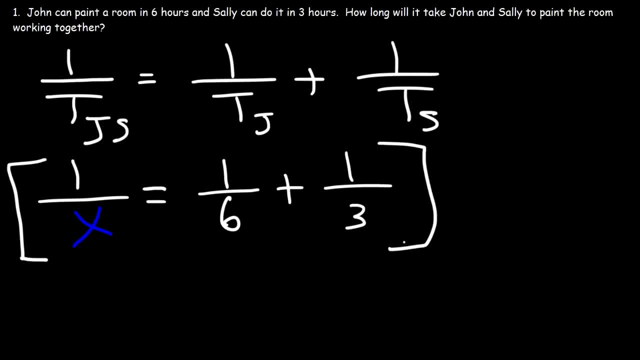 You need to multiply both sides, or basically every fraction in this equation, by something that will get rid of all of the denominators of each fraction. So what we need to do is find out the least common multiple of x, 6.. 6 and 3.. 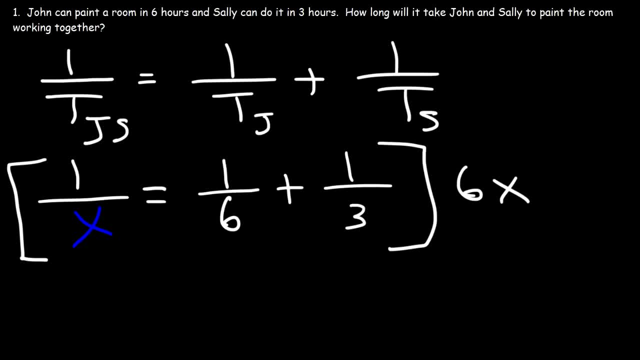 And it's going to be 6x. So let's distribute 6x to everything inside the brackets. So let's multiply 1 over x by 6x. If we do that, the x variable will cancel, and so all we'll get is 6.. 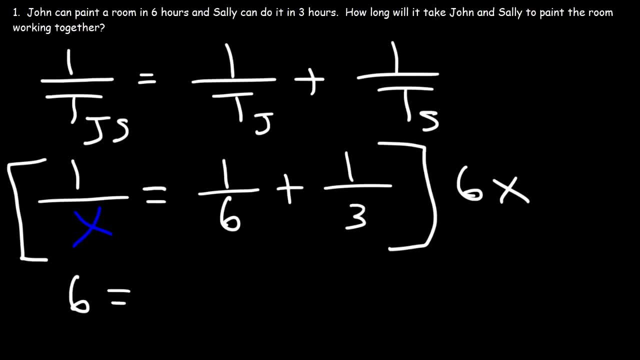 Now, if we multiply these two together, the 6 will be canceled And that will give us x. And then 6x times 1 over 3, or 6x divided by 3. That will give us 2x. 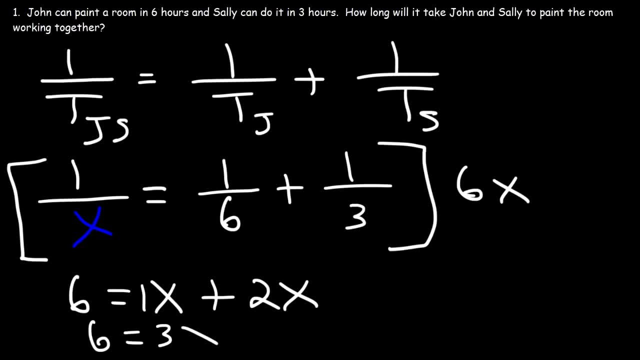 So now we can add 1x plus 2x, which is 3x. At this point we need to divide both sides by 3.. And so x is 6 over 3,, which is 2.. So, working together, it's going to take John and Sally 2 hours to get the answer to this. 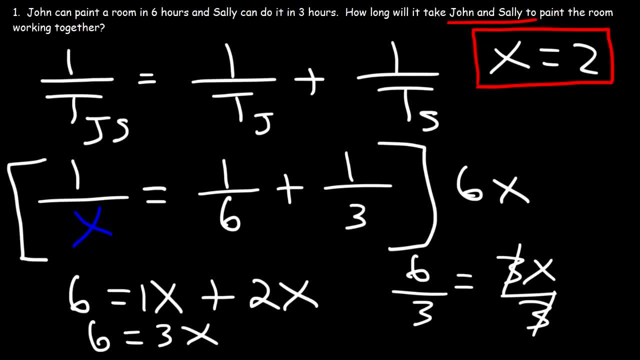 equation, It's going to take 4 hours to paint this room together. Now, for those of you who want to get the answer quickly, here's the formula that you can use: The time it takes for A and B to get the job done working together is going to be 1 over. 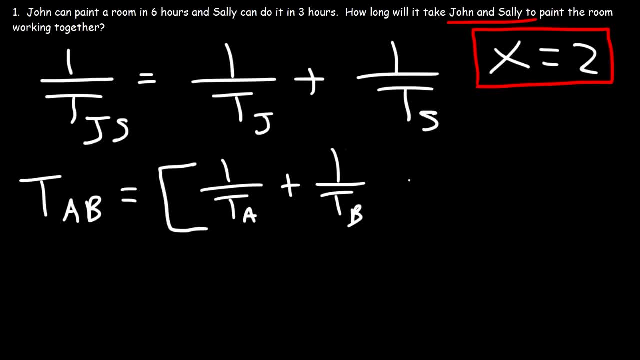 T A plus 1 over T B. All in the brackets or parentheses, Okay, raised to the minus 1.. So in this case, let's say A corresponds to John and B corresponds to Sally. It's simply 1 over 6 plus 1 over 3, raised to the minus 1.. 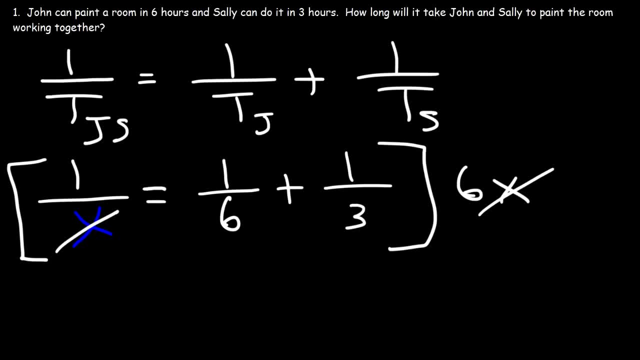 If we do that, the x variable will cancel, and so all we'll get is 6.. Now, if we multiply these two together, the 6 will be canceled, And that will give us x, And then 6x times 1 over 3, or 6x divided by 3.. 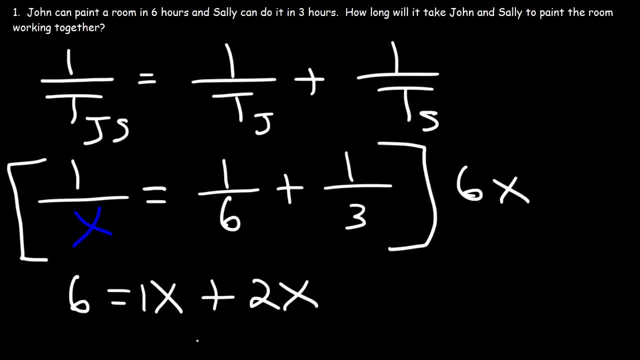 That will give us 2x. So now we can add 1x plus 2x, which is 3x. At this point we need to divide both sides by 3. And so x is 6 over 3,, which is 2.. 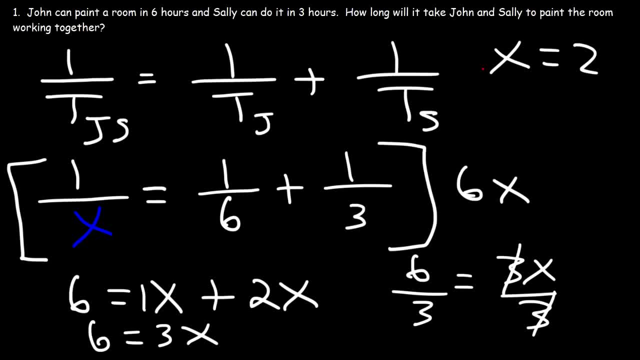 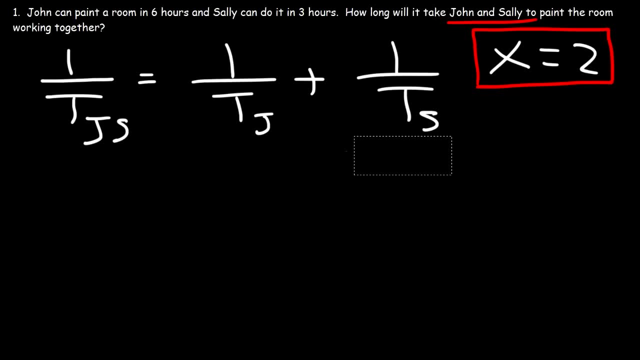 So working together. it's going to take John and Sally 2 hours to get the answer to this equation, And it's also going to take John and Sally 2 hours to paint this room together. Now, for those of you who want to get the answer quickly, here is the formula that you can. 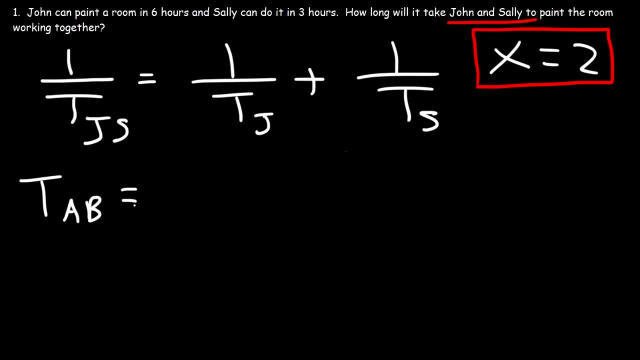 use The time it takes for A and B to get the job done. working together is going to be 1 over tA plus 1 over tB, All in the brackets or parentheses. Okay, And now? what I need to do is I need to add the with the formula to my equation. 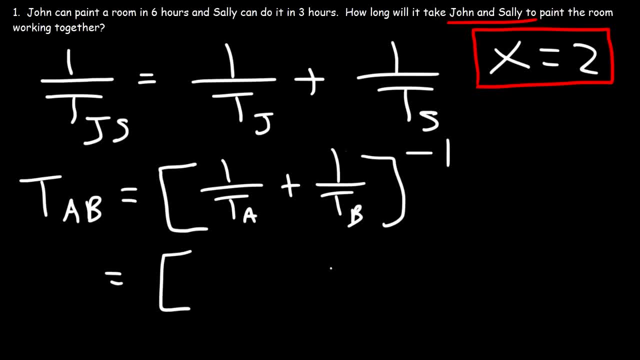 raised to the minus 1.. So in this case, let's say A corresponds to John and B corresponds to Sally. It's simply 1 over 6 plus 1 over 3, raised to the minus 1.. And you can type it into your scientific device and it will give you this answer two. 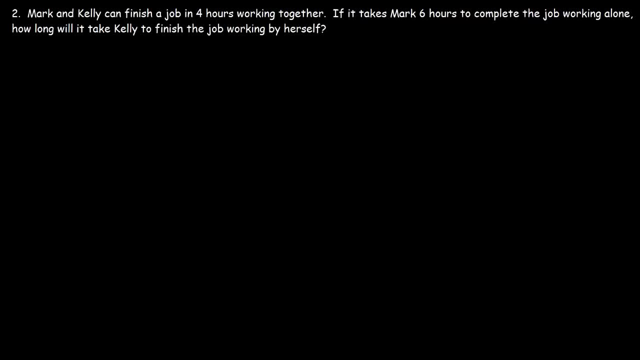 hours. So that's another way in which you could do this problem. Now here is another one. Mark and Kelly can finish a job in four hours working together. If it takes Mark six hours to complete the job working alone, how long will it take? 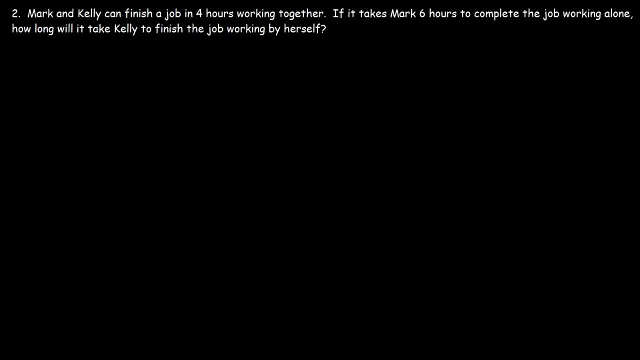 Kelly to finish the job working by herself. So go ahead and try this problem. You could use the same formula. Now I'm going to adjust the subscripts of the formula, So t sub mk. that's the time it takes for Mark and Kelly to get the job done, And. 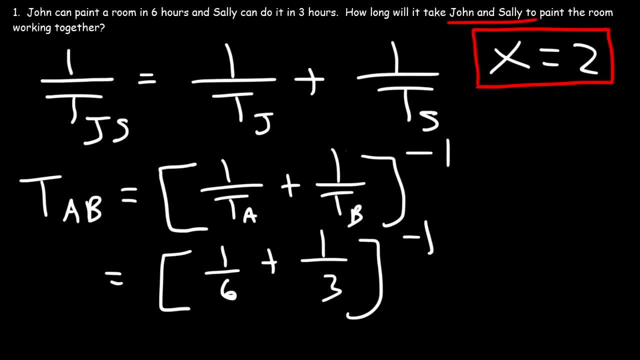 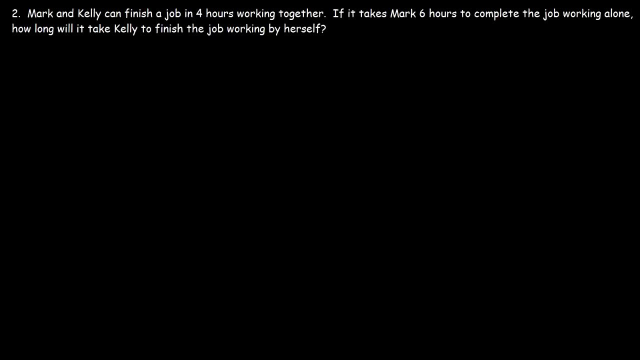 And you could type it into your scientific device and it will give you this answer 2 hours. So that's another way in which you could do this problem. Now here is another one: Mark and Kelly can finish a job in 4 hours working. 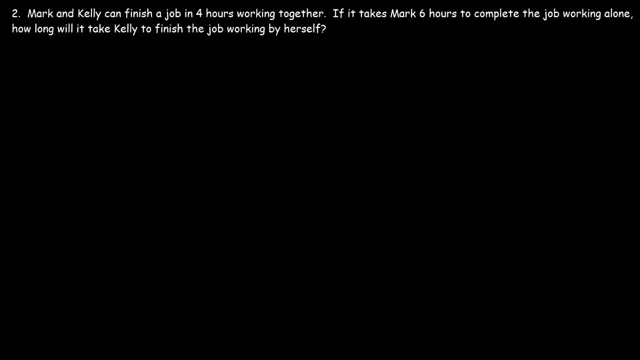 together. If it takes Mark 6 hours to complete the job working alone, how long will it take Kelly to finish the job working by herself? So go ahead and try this problem. You could use the same formula. Now I'm going to adjust the. 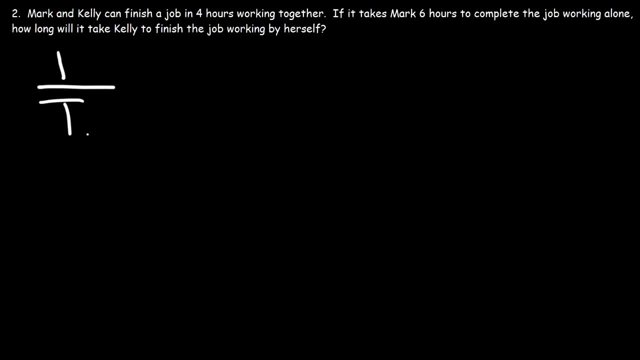 subscripts of the formula. So t sub mk, that's the time it takes for Mark and Kelly to get the job done, And this is going to be equal to 1 over tm. that's for Mark plus 1 over tk, and. 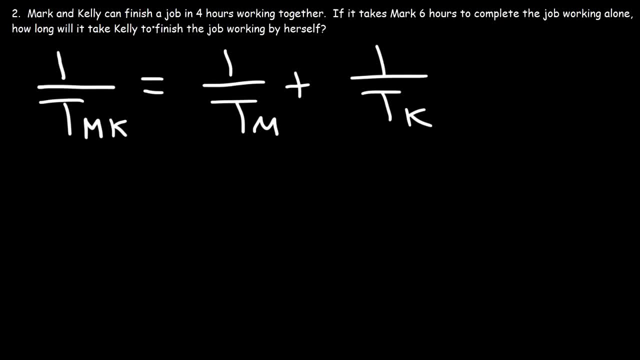 that's for Kelly. So Mark and Kelly can finish the job in 4 hours working together. So t sub mk is 4.. And we know that it takes Mark 6 hours to complete the job working alone. So t sub m is 6.. Our 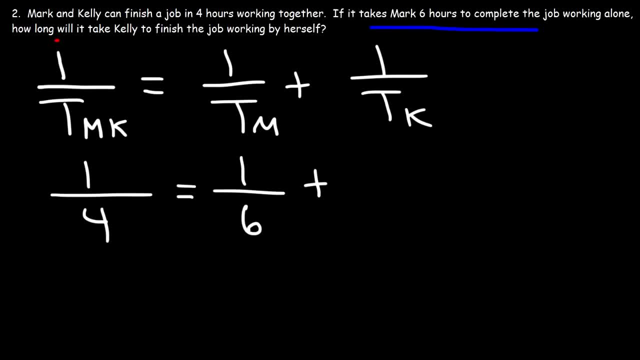 goal is to calculate how long it will take Kelly to finish a job working by herself. So we're looking for the value of tk, So let's call it x. So we're going to use the same process to find the value of x, So let's multiply both sides. 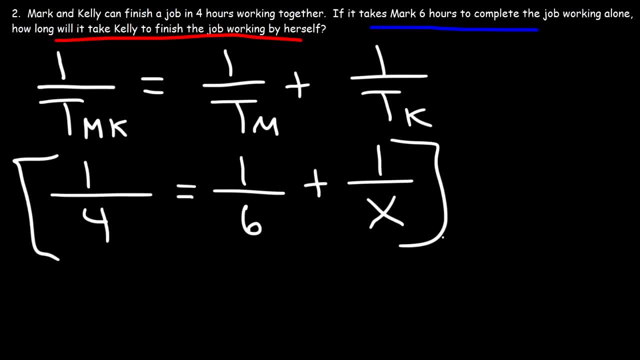 by the LCM or the least common multiple of 4,, 6, and x. Now, if you don't want to find the least common multiple, any multiple will work. You can multiply 4,, 6, and x, which is 24x, and it will help you to get the right answer. But the least. 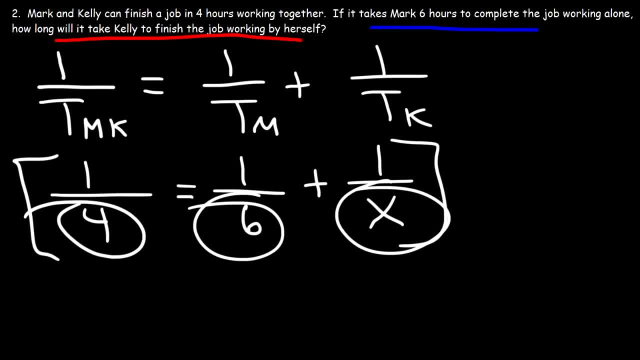 common multiple is 12x, But let's see what happens if we use 24x, Because it's very easy just to multiply what you see here, even though 24x is not the LCM. So 24x times 1 over 4, or 24x divided by 4, that's going to be 6x. 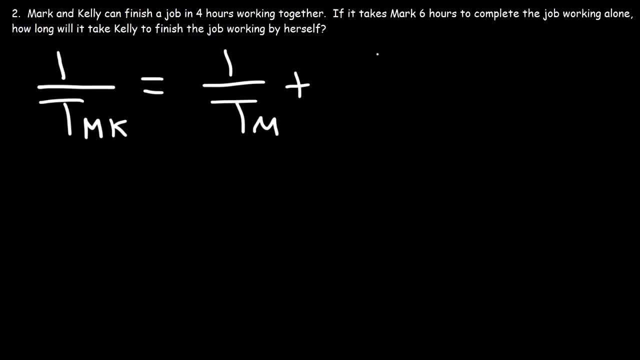 this is going to be equal to 1 over tm, that's for Mark, plus 1 over tk and that's for Kelly. So Mark and Kelly can finish the job in four hours working together. So t sub mk is 4. And we know that it takes Mark. 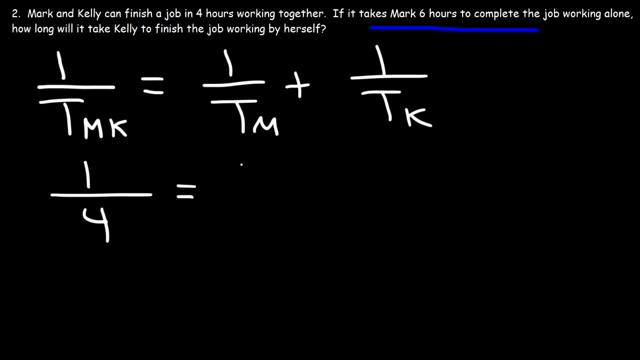 six hours to complete the job working alone. So t sub m is 6.. Our goal is to calculate how long it will take Kelly to finish a job working by herself. So we're looking for the value of tk. So let's call it x. So we're going to use 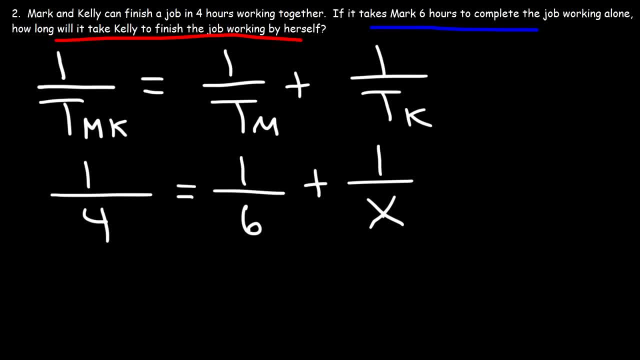 the same process to find the value of x. So let's multiply both sides by the else cm, or the least common multiple of 4,, 6, and x. Now, if you don't want to find the least common multiple, any multiple will work. You can multiply 4,, 6, and x, which. 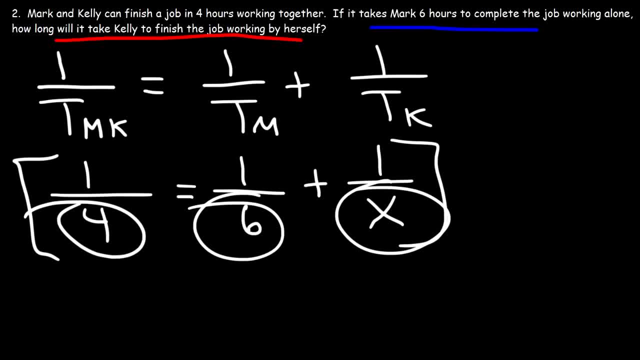 is 24x And it will help you to get the right answer. But the least common multiple is 12x. But let's see what happens if we use 24x, Because it's very easy just to multiply what you see here, even though 24x is not. 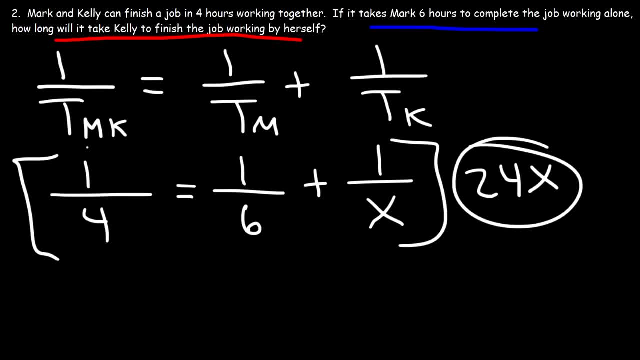 the LCM. So 24x times 1 over 4, or 24x divided by 4, that's going to be 6x, And then 24x divided by 6 is 4x, And then 24x divided by x is simply 24x. 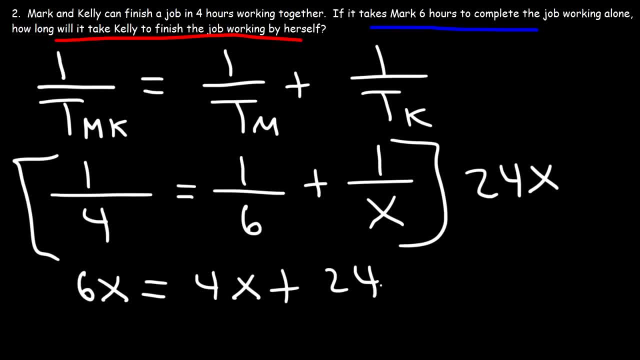 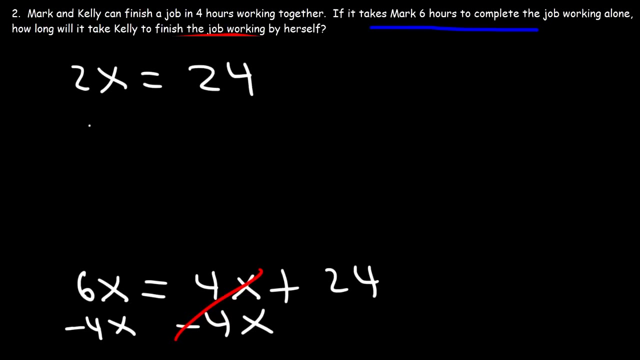 So now let's do some algebra. Let's solve for x. So let's begin by subtracting both sides by 4x. Let's get rid of this, So this will cancel: 6x minus 4x is 2x, and that's equal to 24.. To separate the 2 from the x, let's 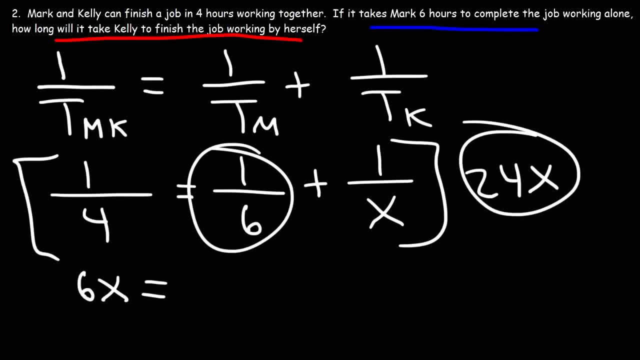 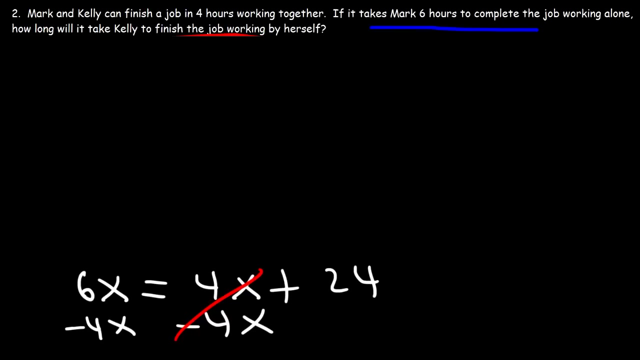 And then 24x divided by 6 is 4x, And then 24x divided by x is simply 24.. So now let's do some algebra. Let's solve for the for x. So let's begin by subtracting both sides by 4x. Let's get rid of this. So this will cancel 6x minus. 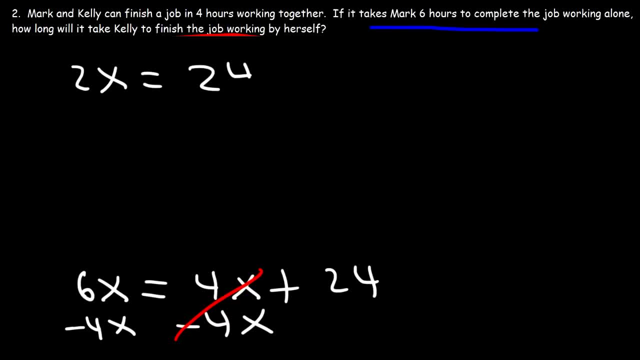 4x is 2x, and that's equal to 24.. To separate the 2 from the x, let's divide both sides by 2.. And so 24 divided by 2 is 12.. So it's going to take Kelly 12 hours to finish. 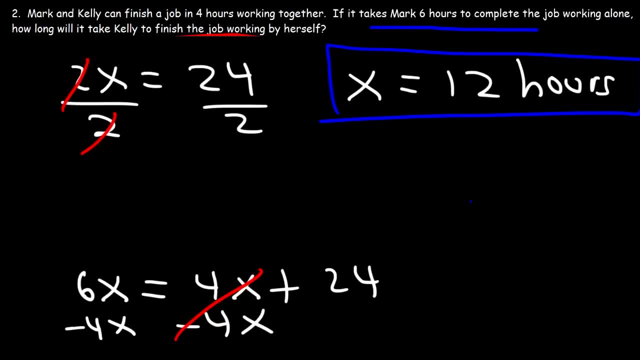 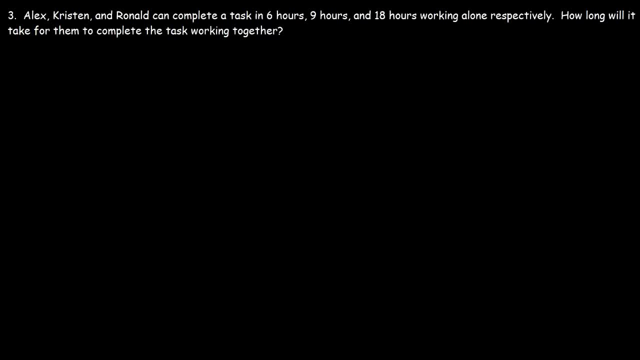 your job working by herself, And so that's all you need to do for this problem. Now let's move on to number 3.. Alex, Kristen and Ronald can complete a task in 6 hours, 9 hours and 18 hours working alone respectively. How long will it take for them to? 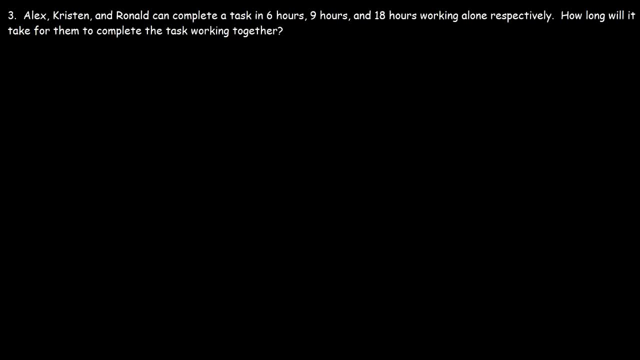 complete the task working together. So this time we have three individuals as opposed to two. So what do you think we need to do? All we need to do is expand the formula. So let's say we have three letters- a, b and c. It's going to be 1 over t a plus 1 over t b, plus 1 over 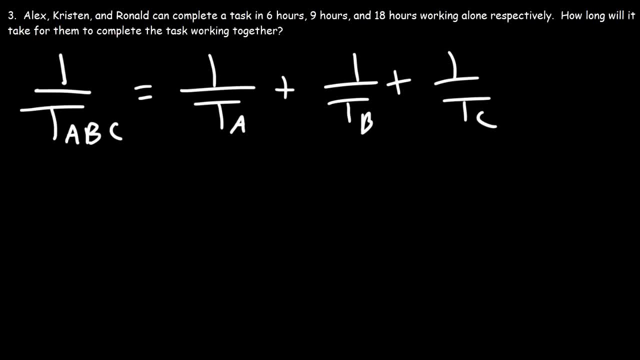 t, c. Now our goal is to find how long is going to take for them to finish a job working together, So we're looking for this variable, So let's replace it with an x. Now: the time it takes Alex to get the job done. 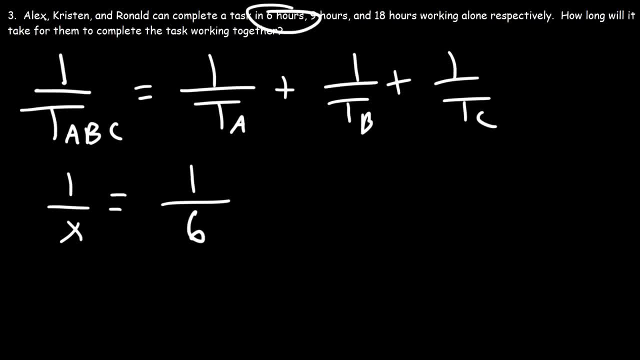 respectively, is going to be the first number because Alex was the first person listed, so that's gonna be six hours. now let's say that B represents Kristen. Kristen can finish it in nine hours and see, we're gonna associate that with Ronald. he can do it in 18 hours. so the math is: 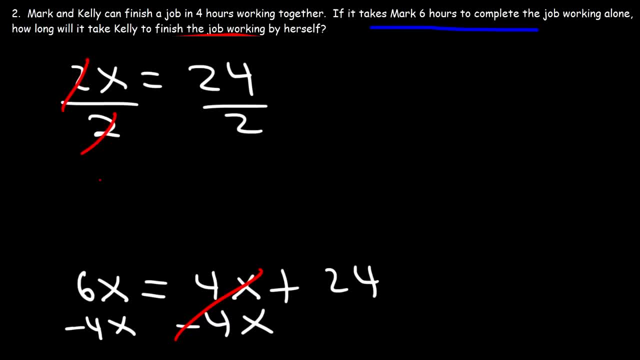 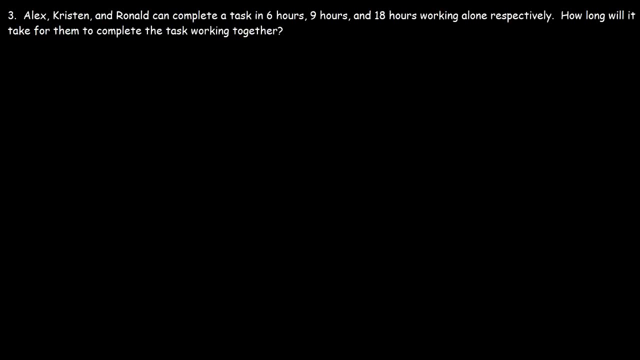 divide both sides by 2.. And so 24 divided by 2 is 12.. So it's going to take Kelly 12 hours to finish the job working by herself, And so that's all you need to do for this problem Now. 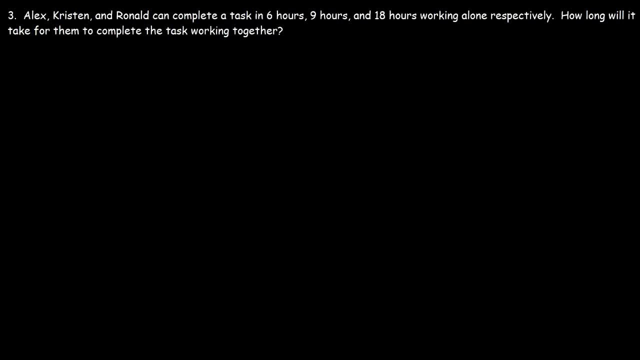 let's move on to number 3.. Alex, Kristen and Ronald can complete a task in 6 hours, 9 hours and 18 hours working alone respectively. How long will it take for them to complete the task working together? 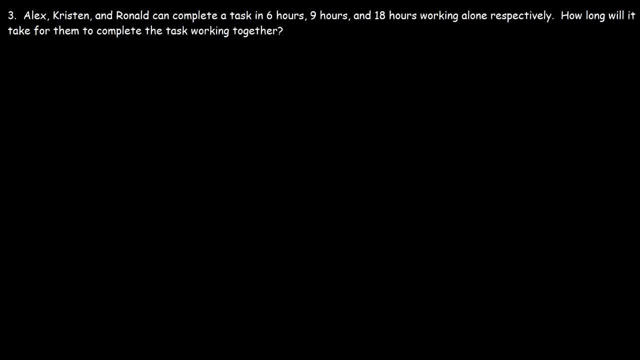 So this time we have three individuals as opposed to two. So what do you think we need to do? All we need to do is expand the formula. So let's say we have three letters: A, B and C. It's going to be 1 over T A plus 1 over T B, plus 1 over T C. 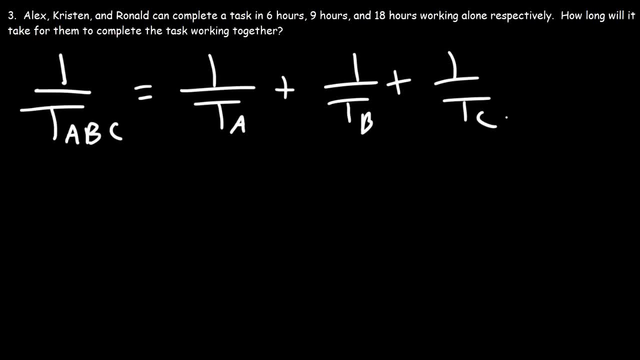 Now our goal is to find how long it's going to take for them to finish the job working together, So we're looking for this variable, So let's replace it with an x. Now, the time it takes Alex to get the job done, respectively, is going to be: 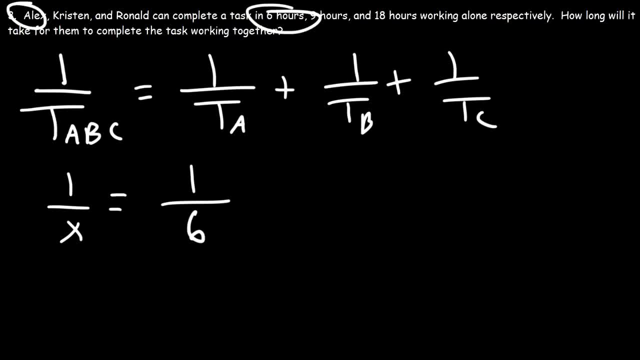 the first number because Alex was the first person listed. So that's going to be 6 hours. Now let's say that B represents Kristen- Kristen can finish it in 9 hours- And C- we're going to associate that with Ronald- He can do it in 18 hours. So the math is going to: 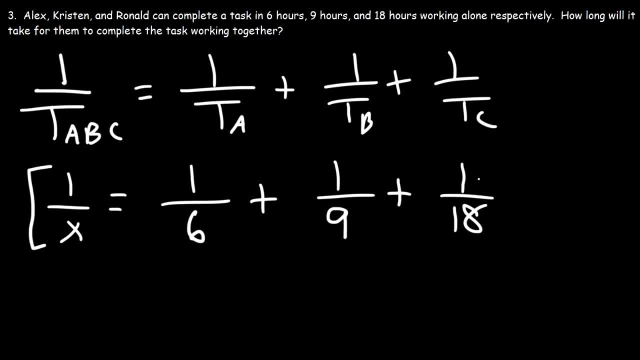 be the same. The only difference is it's simply more work. Now we don't want to multiply x, 9, and 18, and x at the same time, because that's going to give us a very big number. So what is the least common multiple between 6, 9, and 18?? 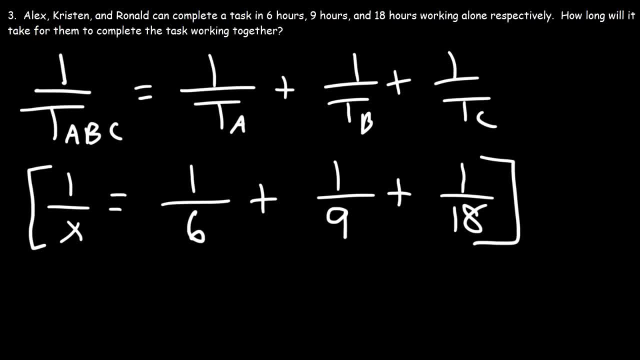 It turns out that it's just 18, because 18 is divisible by 6 and 18 is divisible by 9.. Now to incorporate x as well, the LCM for all four of them will be 18 x 18. x is divisible by. 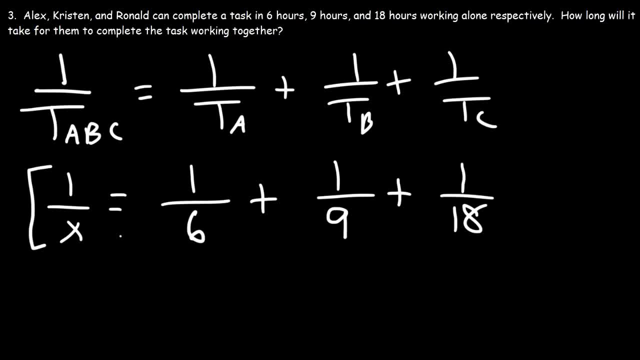 gonna be the same. the only difference is it's simply more work. now we don't want to multiply 6, 9 and 18 and X at the same time, because that's gonna give us a very big number. so what is the least common multiple between 6, 9 and 18? it turns out. 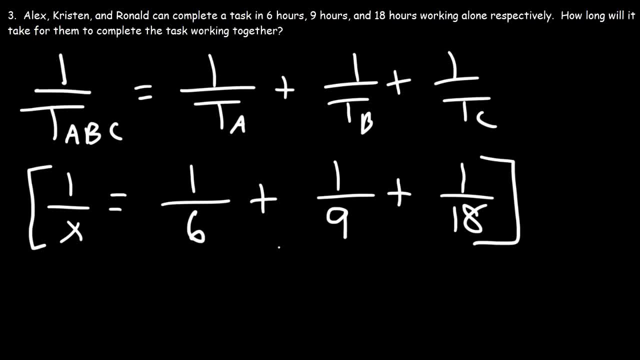 that is just 18, because 18 is divisible by 6 and 18 is divisible by 9. now to incorporate X as well, the LCM for all four of them will be 18 X, 18X, 18X. 18x is divisible by 6,, 9,, 18, and x as well. 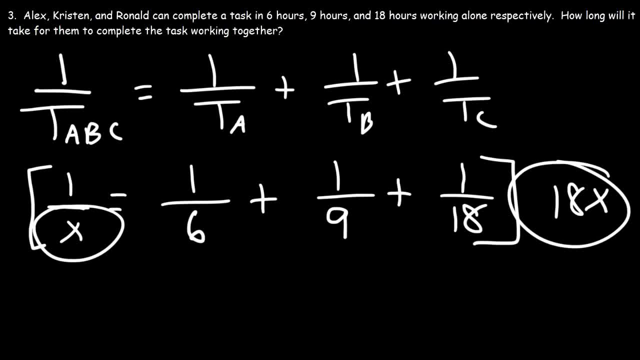 So let's begin by dividing 18x by x, and so that's going to give us 18, and then, if we take that, divide it by 6,, that will give us 3x, and then 18x divided by 9 is 2x, and 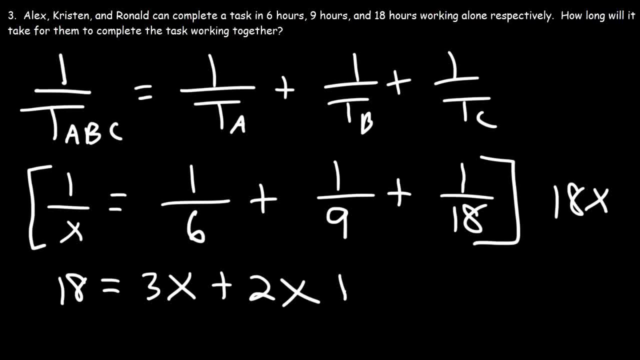 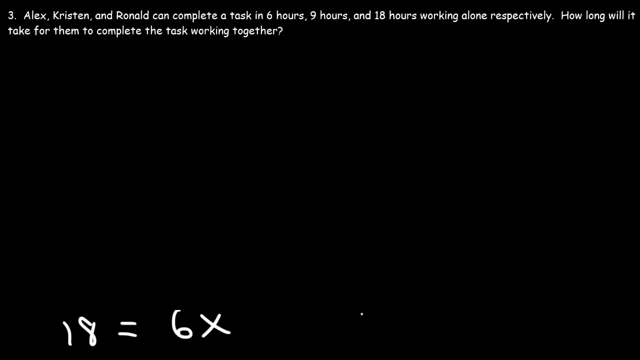 then 18x divided by 18, that's simply x. So 3x plus 2x plus 1x, that's going to be 6x. Now let's divide both sides by 6.. 18 divided by 6 is 3.. 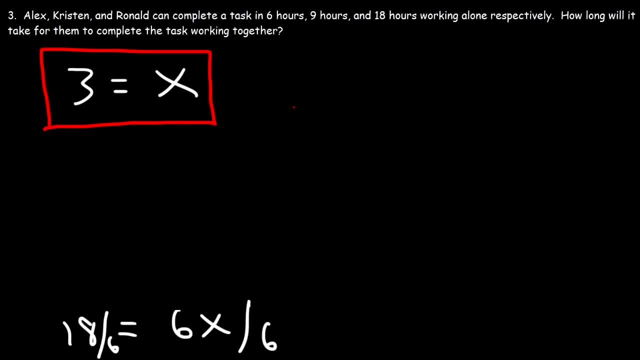 So it's going to take them 3 hours for all 3 of them To complete the task working together, And that's basically it for this problem. That's all you need to do to get the answer. As you can see, it's not that bad. 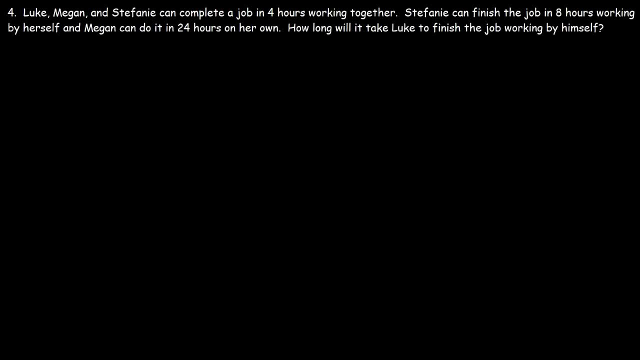 Now let's move on to the next one. Luke, Megan and Stephanie can complete a job in 4 hours working together. Stephanie can finish the job in 8 hours working by herself, And Megan can do it in 24 hours On her own. 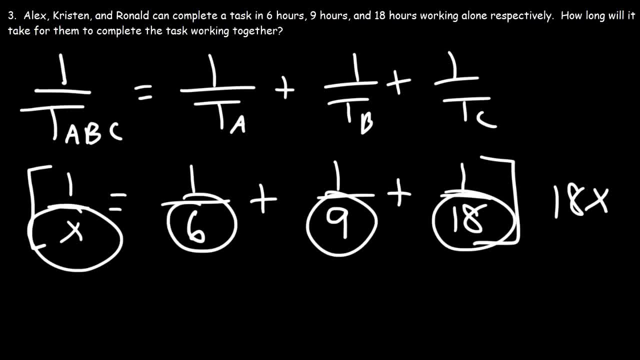 6,, 9,, 18, and x as well. So let's begin by dividing 18x by x, and so that's going to give us 18, and then, if we take that, divide it by 6,, that will give us 3x and then 18x. 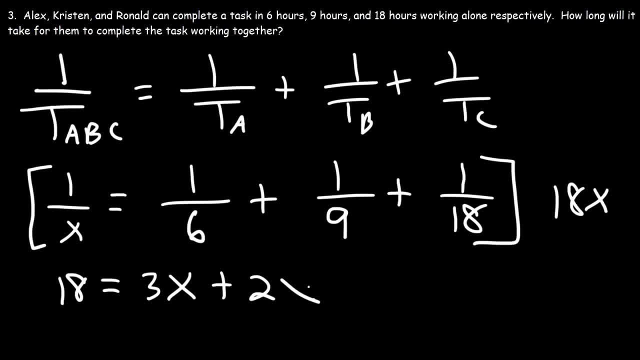 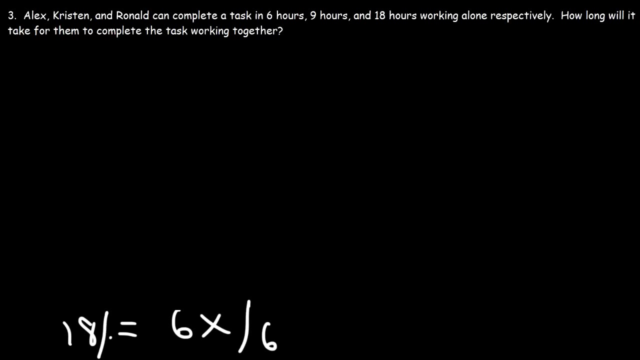 divided by 9 is 2x, and then 18x divided by 18, that's simply x. So 3x plus 2x plus 1x, that's going to be 6x. Now let's divide both sides by 6.. 18 divided by 6 is 3.. 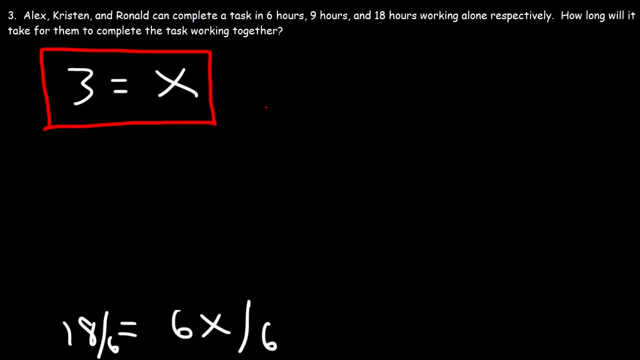 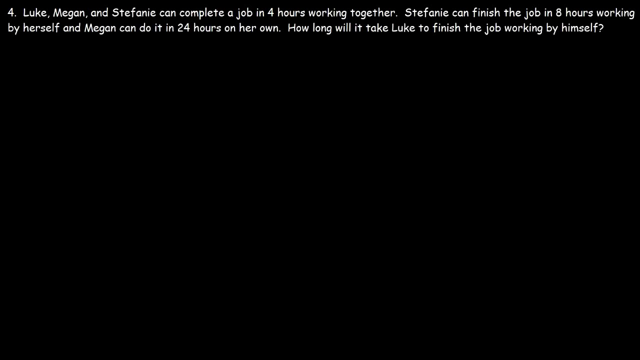 So it's going to take them 3 hours for all 3 of them to complete the task working together, And that's basically it for this problem. That's all you need to do to get the answer. As you can see, it's not that bad. Now let's move on to the next one: Luke, Megan and. 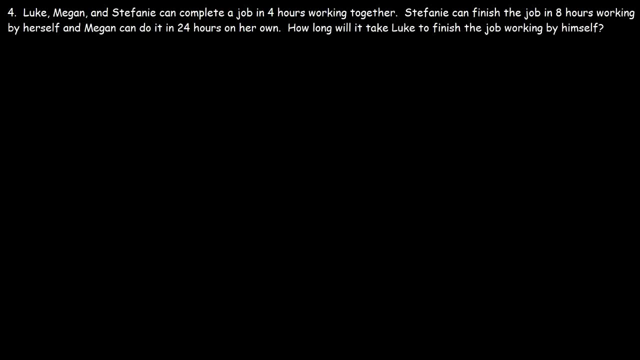 Stephanie can complete a job in 4 hours working together. Stephanie can finish the job in 8 hours working by herself, And Megan can do it in 24 hours on her own. How long will it take Luke to finish the job working by himself? 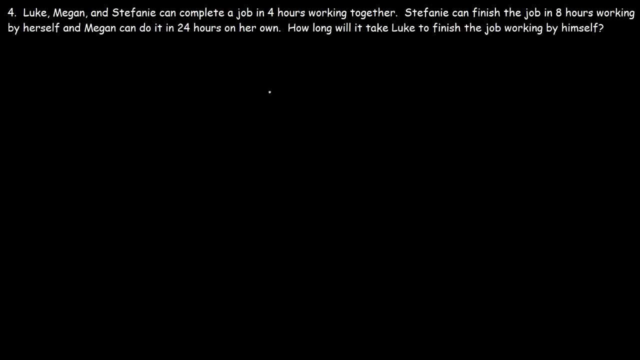 So once again, we have 3 individuals, and we're going to use this formula again. So, working together, all 3 of them can finish the job in 4 hours. Now Stephanie can do the job in 8 hours, So let's say, A corresponds to Stephanie and Megan can do it in 24 hours. So we're going to 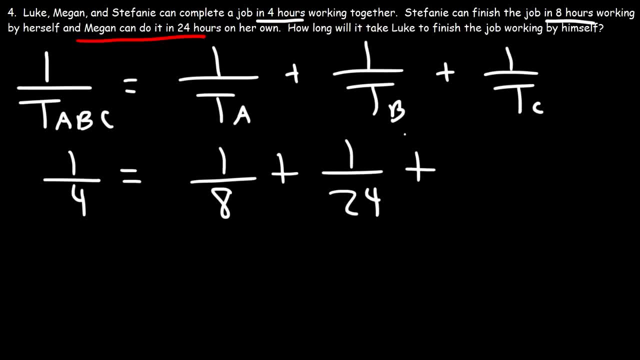 make B correspond to Megan, And let's represent C with Luke. How long will it take Luke to finish the job working by himself? So let's replace TC with X. So let's find the LCM of 4,, 8,, 24, and X. So what do you? 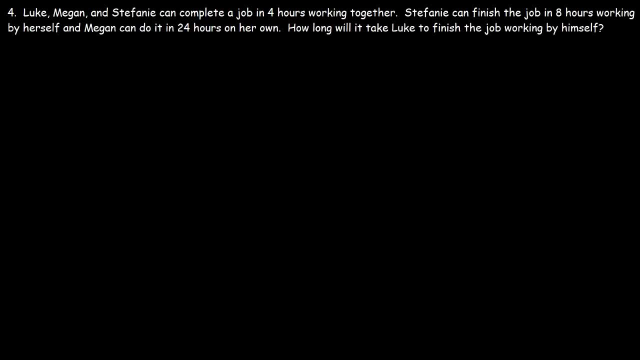 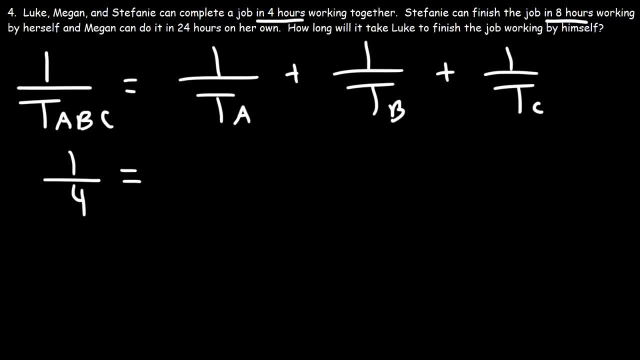 Now, Stephanie can do the job in 8 hours, So let's say A corresponds to Stephanie And Megan can do it in 24 hours. So we're going to make B correspond to Megan And let's represent C with Luke. How long will it take Luke to finish the job, working by himself? 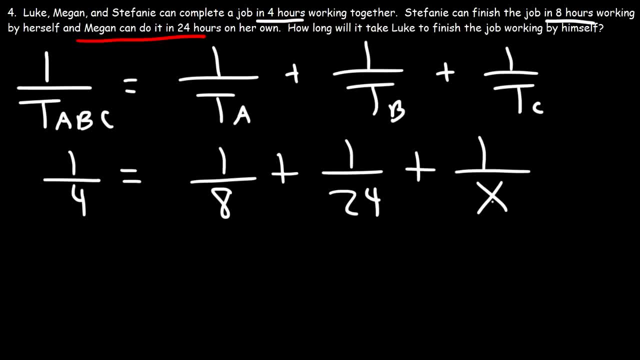 So let's replace TC with X. AndικήHH Ki då bait. We didn't produce C 2C. We don't replace TC with L If, And then 24x divided by 8 is 3x, And then 24x divided by 24 is simply x. 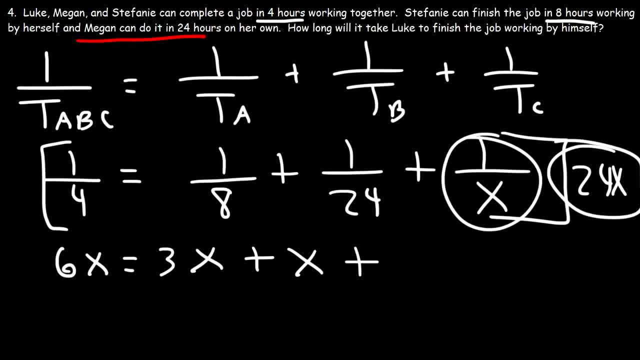 And finally, 24 divided by x is 24.. So let's go ahead and combine like terms: 3x plus 1x is 4x. So we have: 6x is equal to 4x plus 24.. And then let's subtract both sides by 4x. 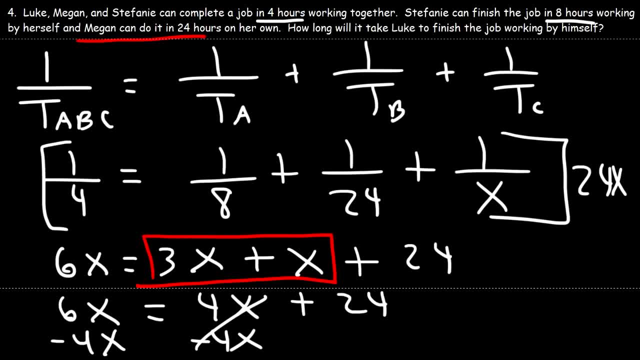 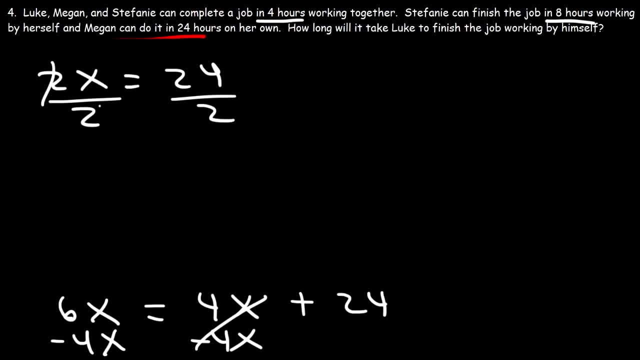 This equation looks very familiar: 6x minus 4x is 2x, And then we're going to divide by 2.. And so x is 12.. Which means that it's going to take Luke 12 hours to finish the job, working by himself. 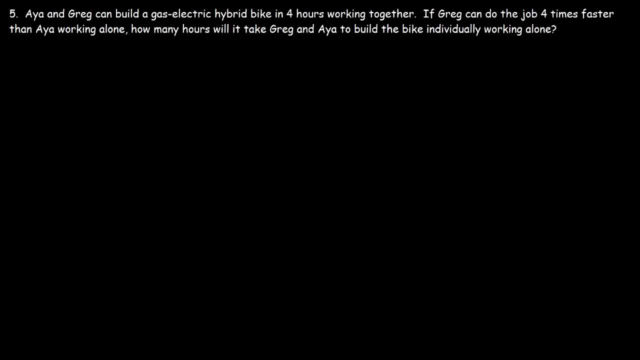 And that's the answer for this problem. Now the next problem Is going to be a little more difficult: Number 5. Aya and Greg can build a gas electric hybrid bike in 4 hours working together, If Greg can do the job 4 times faster than Aya working alone. 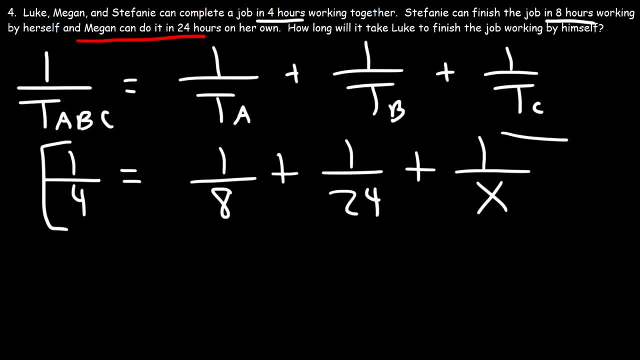 think it's going to be. Notice that 4 and 8, they can go into 24.. So it turns out that the least common multiple is going to be 24X. So if we divide 24X by 4, we're going to get. 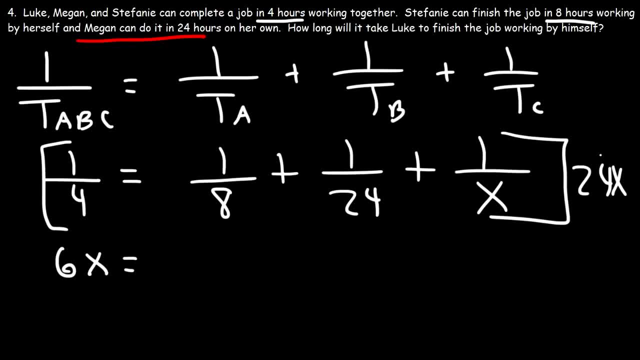 6X, That's going to give us 6X, And then 24X divided by 8 is 3X, And then 24X divided by 24 is simply X, And finally, 24 divided by X is 24.. 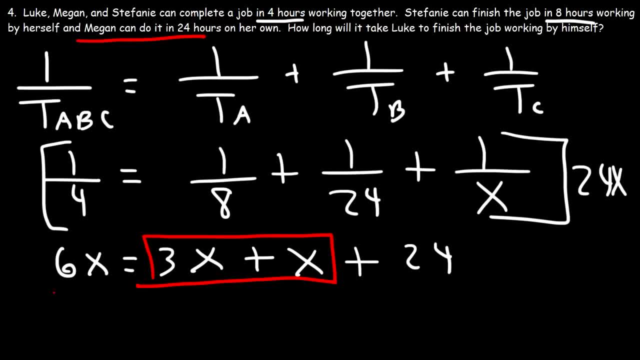 So let's go ahead and combine like terms: 3X plus 1X is 4X, So we have: 6X is equal to 4.. So let's go ahead and combine like terms: 3X plus 1X is 4X, So we have 6X is equal to. 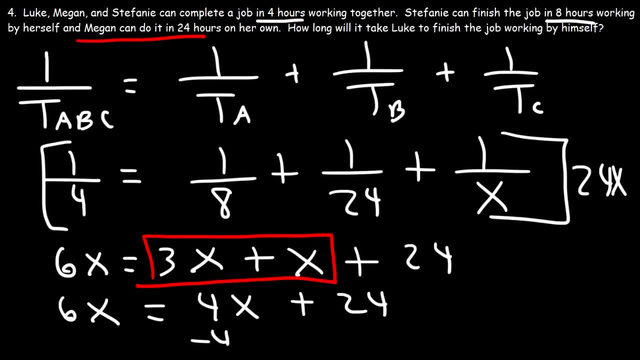 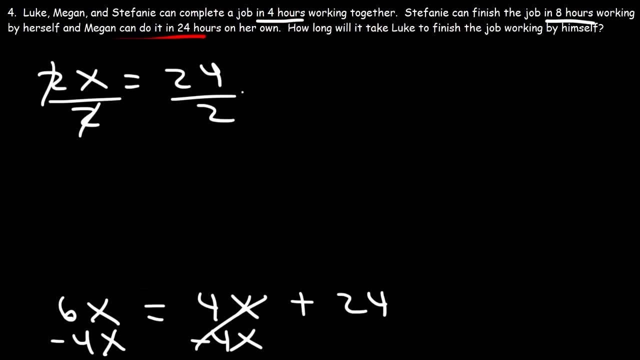 4X plus 24.. And then let's subtract both sides by 4X. This equation looks very familiar: 6X minus 4X is 2X, And then we're going to divide by 2. And so X is 12.. Which means that: 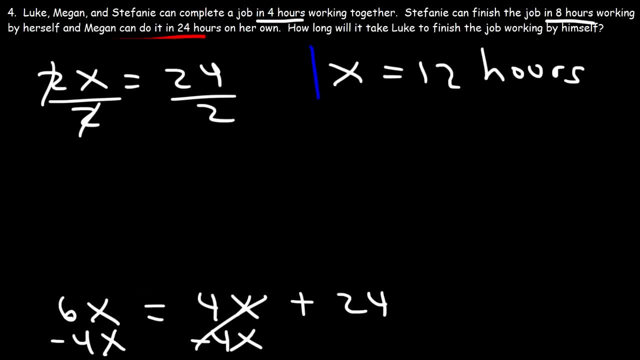 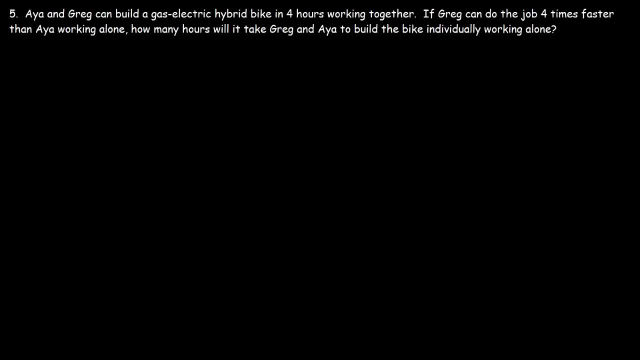 it's going to take Luke 12 hours to finish the job working by himself. And that's the answer for this problem. Now the next problem is going to be a little more difficult: Number 5. Aya and Greg can build a gas-electric hybrid bike in 4 hours working together If 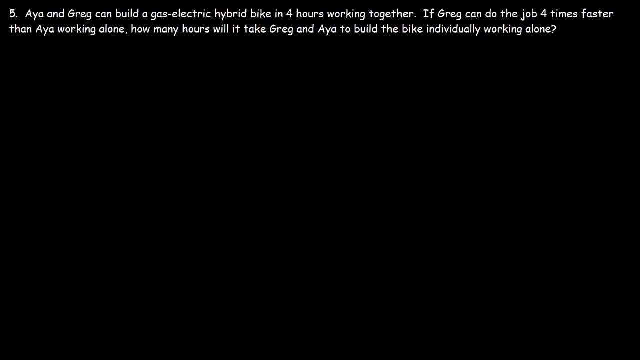 Greg can do the job 4 times faster than Aya working alone. how many hours will it take Greg and Aya to build a bike individually working alone? So go ahead and try that problem. So we're going to have T sub A and G instead of B. So T sub A is going to be the time it. 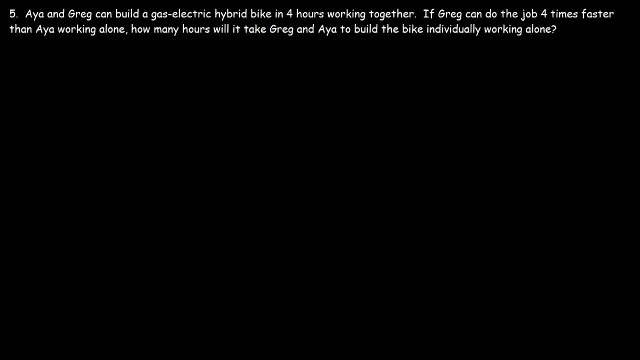 How many hours will it take Greg and Aya to build a bike individually working alone? So go ahead And try that problem. So we're going to have T sub A and G instead of B. So T sub A is going to be the time it takes for Aya to get the job done. 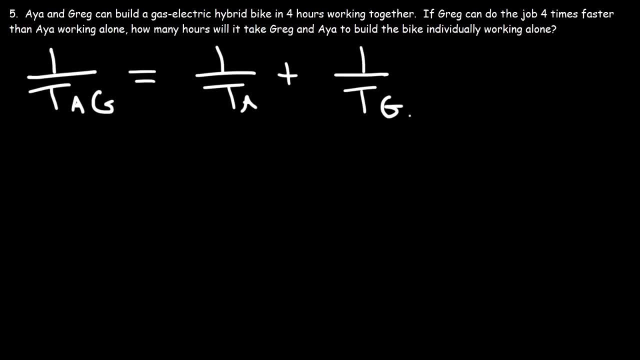 And T sub G is for Greg. Now how can we incorporate this sentence into the problem? Greg can do the job 4 times faster than Greg, And Greg can do the job 4 times faster than Aya working alone. So what does that mean in terms of hours? 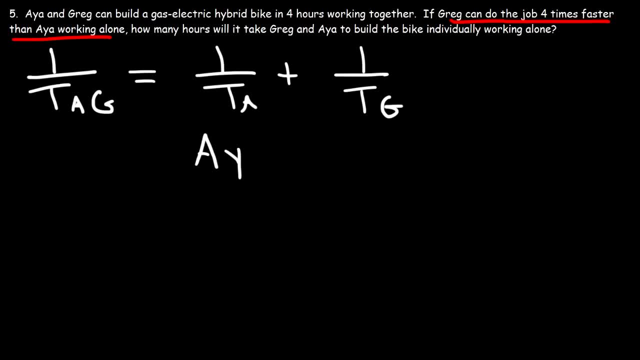 Well, let's slow it down a little bit And think about it. So let's write down Aya and Greg. So let's say, if Aya can finish the job in 8 hours Now, if Greg could do the job 4 times faster than Greg. 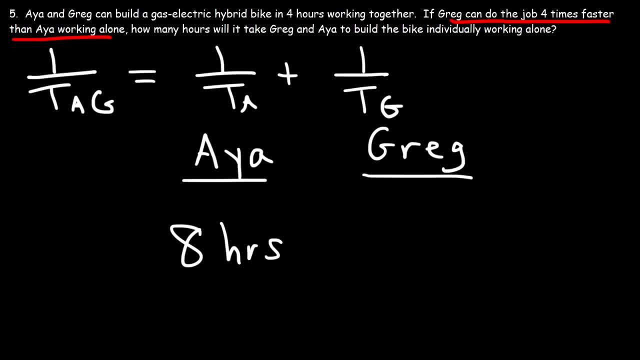 Now, if Greg can do the job 4 times faster than Greg. Now, if Greg can finish the job in 8 hours, Now, if Greg can do the job 4 times faster than Greg, faster than Aya working alone, how many hours will it take Greg to get the job done if Aya? 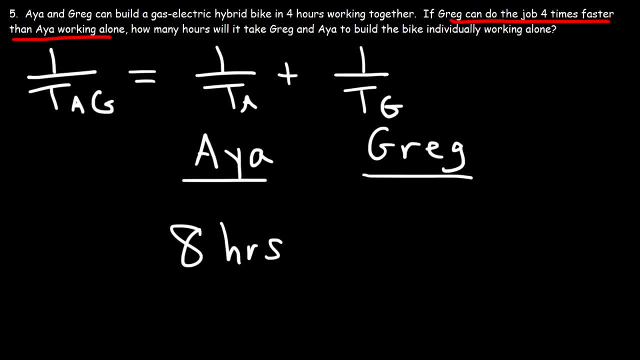 can do it in 8 hours. Should we multiply by 4 and say it's going to take him 32 hours, Or should we divide by 4 and say it's going to take him 2 hours? Now, based on the sentence or the problem, rather, Greg can do the job faster than Aya. 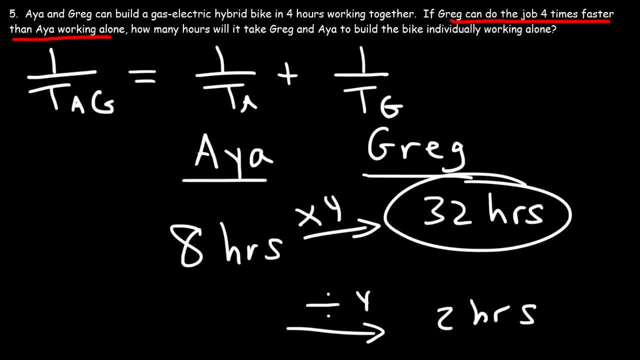 If it takes him 32 hours to get it done, he's not working faster, he's working slower. So therefore, it will take Greg 2 hours to get it done if Aya can do it in 8 hours. So what does that mean? 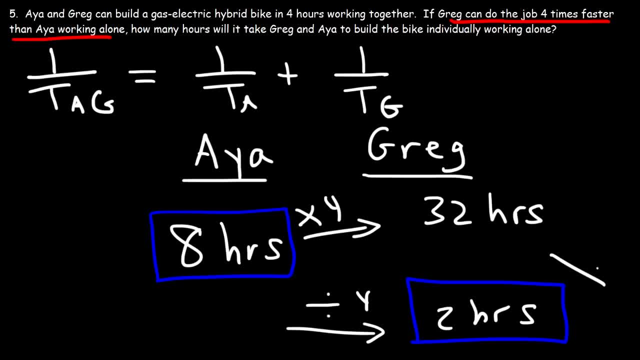 So let's say: if it takes Greg X hours, Okay, to get the job done, That means it's going to take Aya four times X, because it's going to take her four times longer, since she's working four times slower than Greg. So let's apply this information. 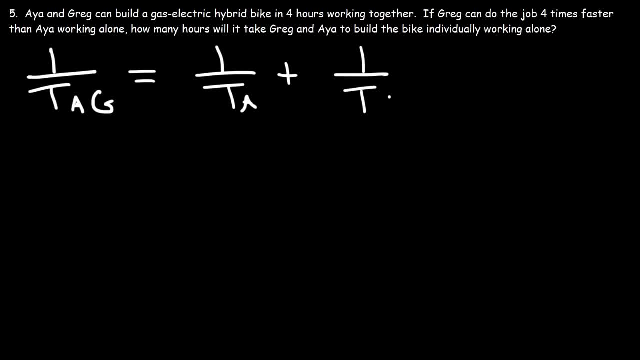 takes for Aya to get the job done And T sub G is for Greg. Now how can we incorporate this sentence into the problem? Greg can do the job 4 times faster than Aya working alone. So what does that mean in terms? 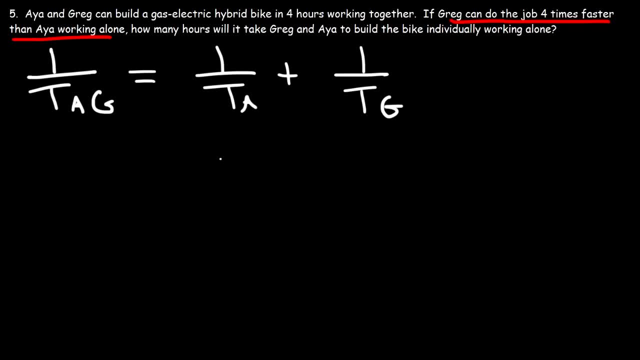 of hours. Well, let's slow it down a little bit and think about it. So let's write down Aya and Greg. So let's say, if Aya can finish the job in 8 hours Now, if Greg could do the job 4 times faster than Aya working alone, how many hours will it? 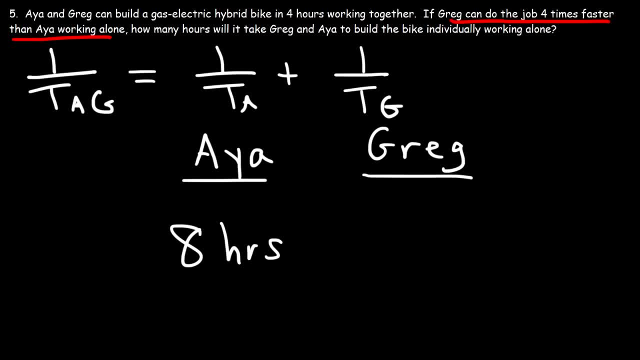 take Greg to get the job done. if Aya can do it in 8 hours, Should we multiply by 4 and say it's going to take him 32 hours? Or should we divide by 4 and say it's going to take him 2 hours? 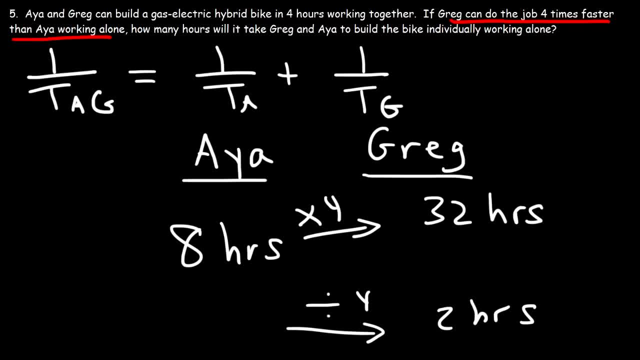 Now, based on the sentence or the problem. rather, Greg can do the job faster than Aya. if it takes him 32 hours to get it done, he's not working faster, he's working slower. so therefore, it will take Greg two hours to get it done. 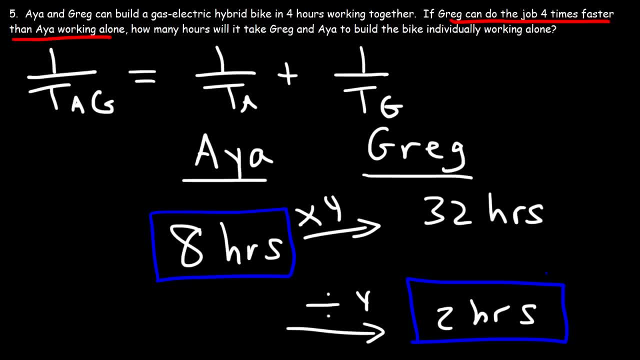 if Aya can do it in 8 hours. So what does that mean? So let's say, if it takes Greg x hours to get the job done, That means it's going to take Aya 4 times X, because it's gonna take her four times longer since she's working four. 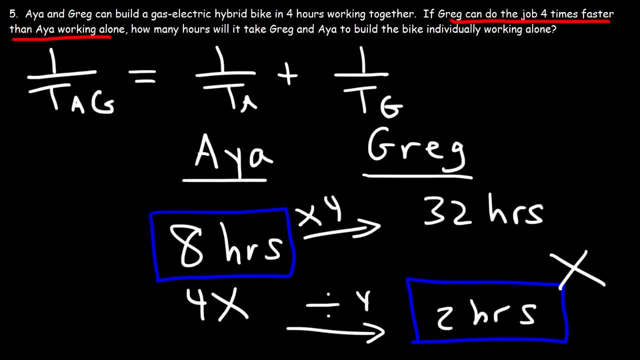 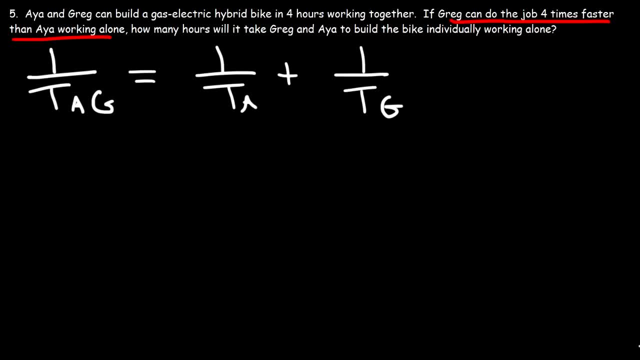 times slower than Greg. so let's apply this information. so our goal is to find out how many hours it will take Greg and Aya to build a bike individually working alone. so we're gonna say that it takes Greg X hours to get the job done, Aya. 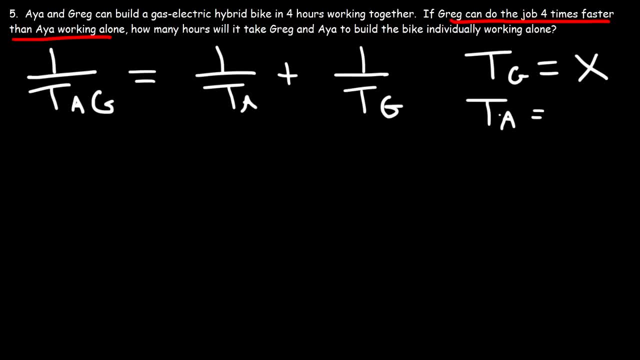 who's working four times slower, it's gonna take her four times longer or four acts to get it done. now, working together, they can build it in four hours. so that's TAG. let's replace that with four. TA is going to be four, X, TG is going to be X. 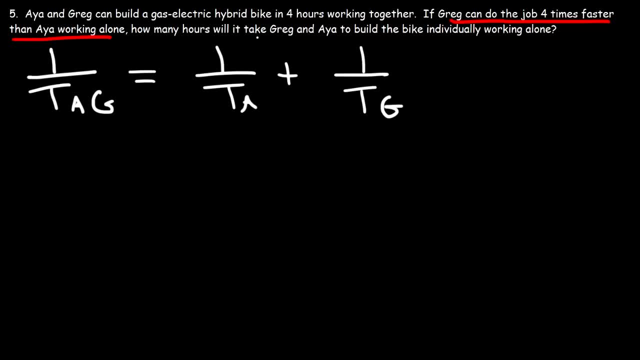 So our goal is to find out how many hours it will take Greg and Aya to build a bike individually, working alone. So we're going to say that it takes Greg X hours to get the job done. Aya, who's working four times slower, it's going to take her four times longer, or four X, to get it. 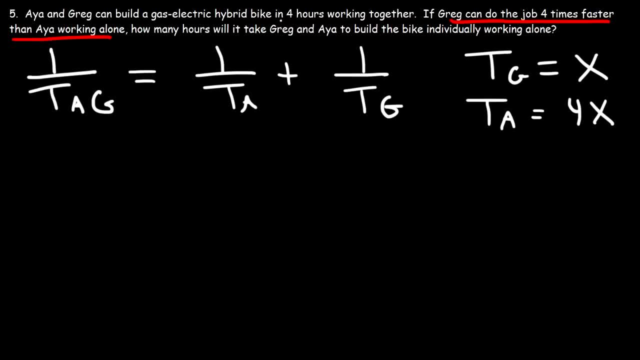 done Now. working together, they can build it in four hours. So that's TAG. Let's replace that with four. TA is going to be four, X, TAG is going to be X. So now we have the equation. Let's solve for the value of X. 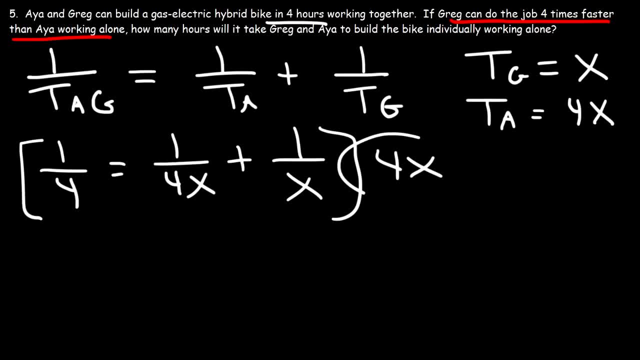 So let's multiply both sides by four X. Four X divided by four is X, and four X divided by itself, That's going to be one And four X divided by X is four, And so X is simply one plus four, which is four X. So now we have the equation. So now we're going to solve for the value of X. 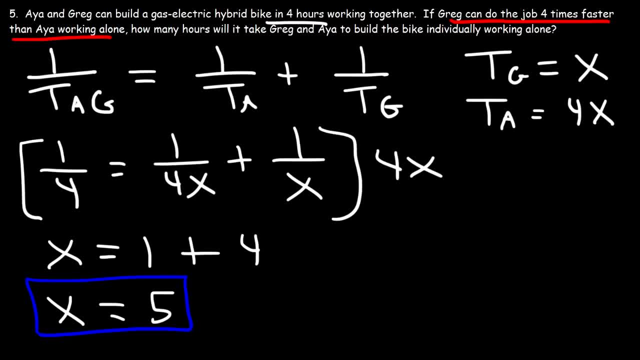 or five. So now that we have the value of x, all we need to do is plug it in to those two expressions. Now the time that it takes Greg to get it done is equal to x. so that's going to be five hours, And the time that it takes Aya to get the job done is four times. 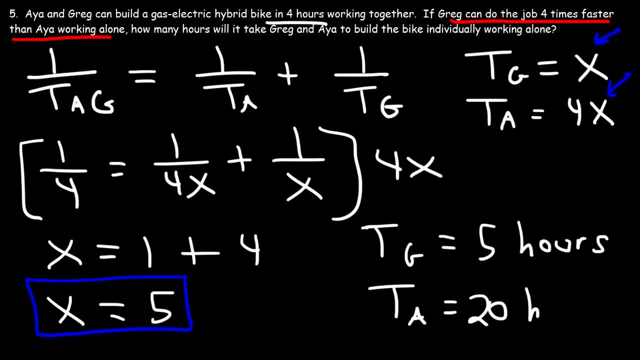 x or four times five, which is twenty hours, And of course you can confirm that this is correct by using this formula. It's going to be one over five plus one over twenty raised to the minus one. So go ahead and type that into your scientific calculator and that. 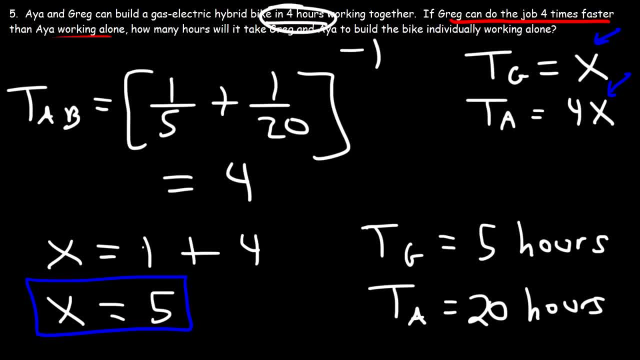 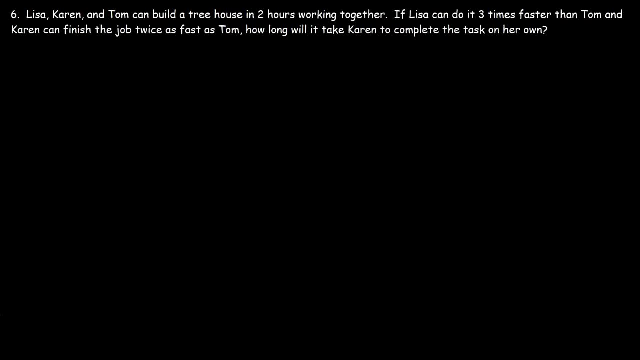 will give you four. So these are the answers to the problem. That's the time it's going to take for Aya and Greg to build it working individually alone. Number six: Lisa, Karen and Tom can build a tree house in two hours working together If Lisa can do it three times faster than Tom and 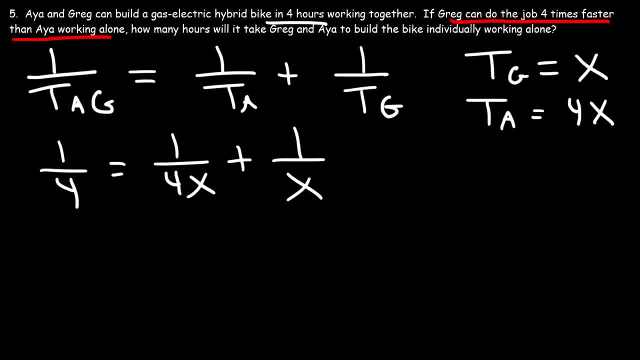 So now we have the equation, Let's solve for the value of x. So let's multiply both sides by 4x. 4x divided by 4 is x, and 4x divided by itself, that's going to be 1.. 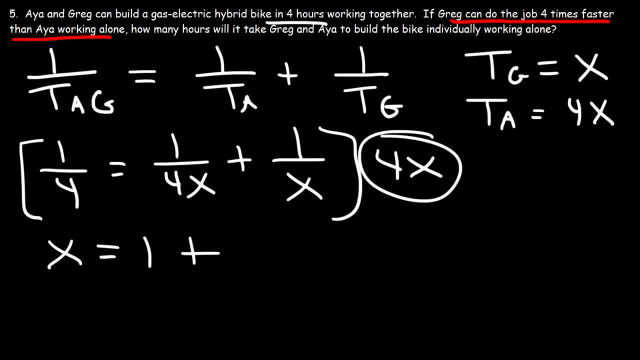 And 4x divided by x is 4. And so x is simply 1 plus 4, or 5.. So now that we have the value of x, all we need to do is plug it in to those two expressions. Now, the time that it takes Greg to get it done is equal to x, so that's going to be 5 hours. 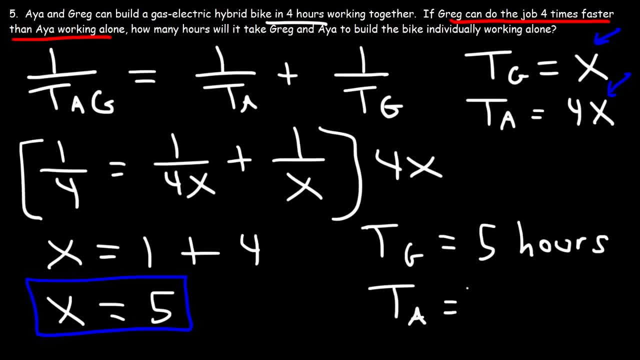 And the time that it takes Aya to get the job done is 4 times x or 4 times 5, which is 20 hours. And, of course, you can confirm that this is correct By using the equation, Using this formula: 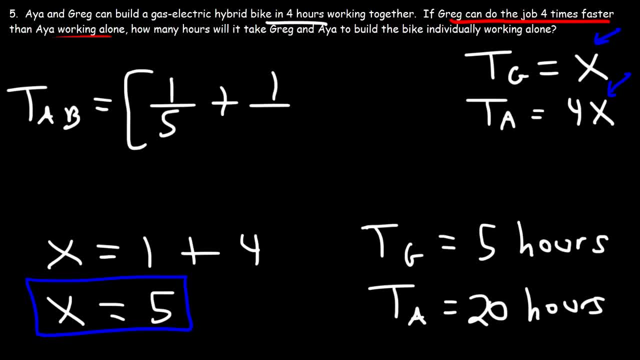 It's going to be 1 over 5 plus 1 over 20, raised to the minus 1.. So go ahead and type that into your scientific calculator And that will give you 4.. So these are the answers to the problem. 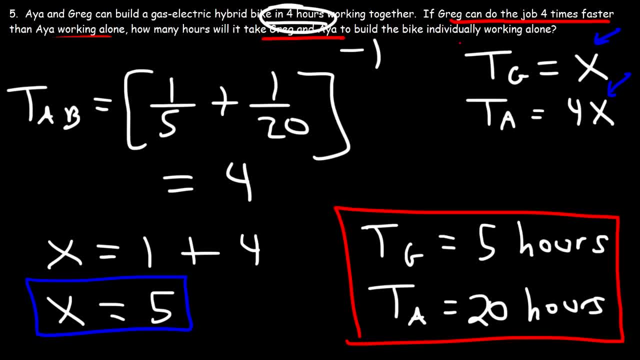 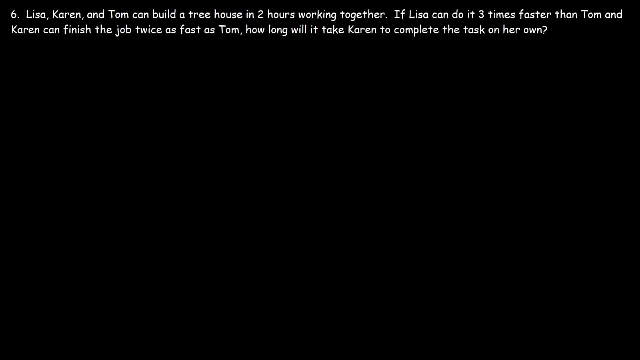 That's the time it's going to take Aya and Greg to build it. They can do it without working individually alone. Number 6. Lisa, Karen and Tom can build a tree house in two hours working together. If Lisa can do it three times faster than Tom, and Karen can finish the job twice as fast as Tom. 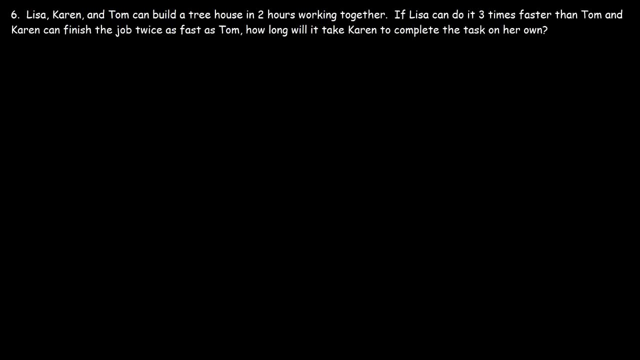 how long will it take Karen to complete the task on her own? So that's number 3.. So let's write Lisa, Karen and Tom. So Lisa can do it three times faster than Tom. So thinking about it in the reverse direction, Tom is three times slower than Lisa, which means Tom is going to take three times longer than Lisa. 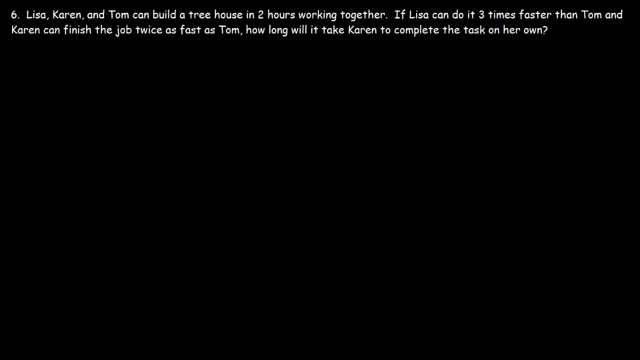 Karen can finish the job in twenty hours, then there's a three-hour time frame to complete the task And that if we do it three times faster than Tom and Karen can finish the twice as fast as Tom, how long will it take Karen to complete the task on her own? 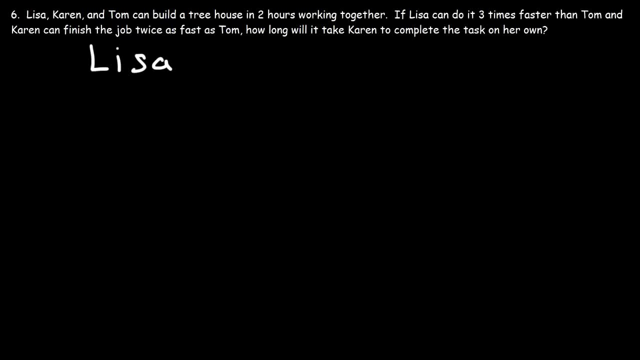 So let's write Lisa, Karen and Tom. So Lisa can do it three times faster than Tom. So thinking about it in the reverse direction, Tom is three times slower than Lisa, which means Tom is gonna take three times longer than Lisa. 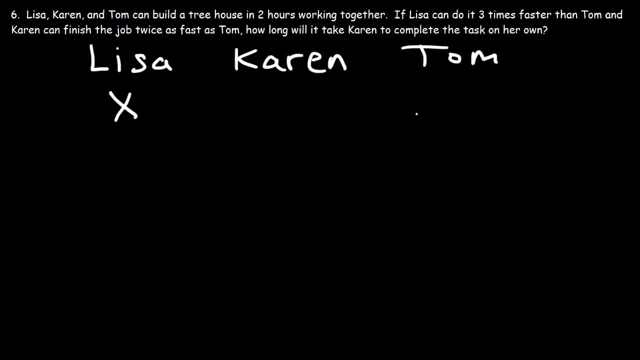 So if Lisa takes X hours, Tom is gonna take three times X hours to get the job done. Now what about Karen? Karen can do the job twice as fast as Tom, which means Tom is twice as slow as Karen. So if Karen could do it in X hours? 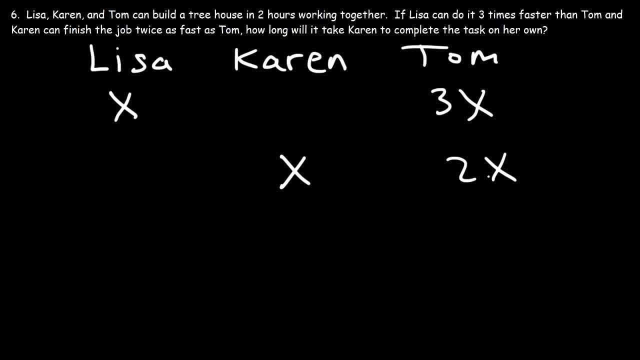 Tom can do it in two X hours or twice as long. But now we can't have two different values for Tom, nor can we have the same value for Lisa and Karen. So how do we make this work? What do we need to do here? 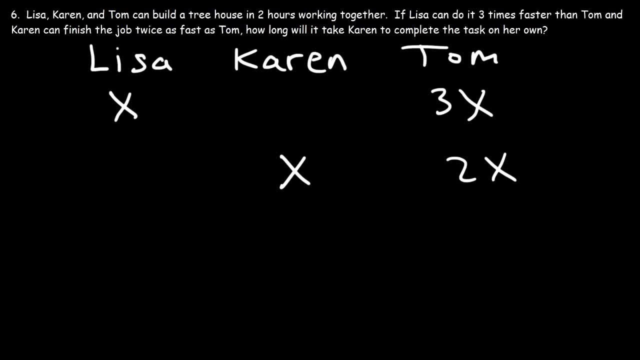 Hmm, Take a minute and try to figure it out. Pause the video and see if you can get the answer Now. somehow we need to make these two values the same. Now let's analyze this situation. If we divide both of those values by three, 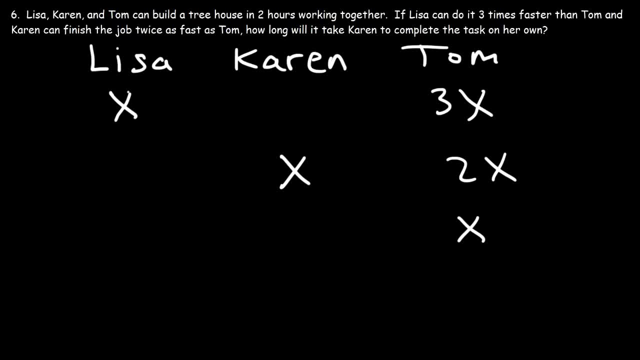 three. X divided by three will be X, and X divided by three will be X over three. Now let's do the same for Tom and Karen, but we're gonna divide it by two. Two X divided by two will give us X, and X divided by two is just X over two. 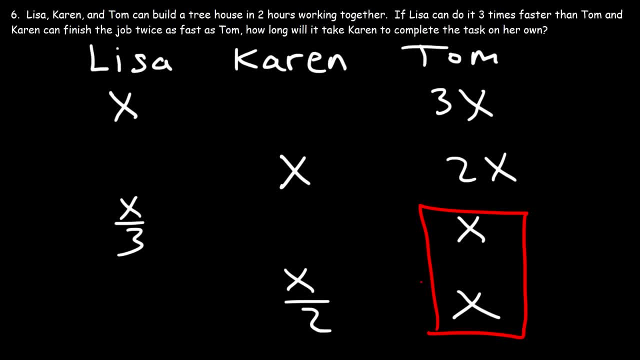 And so now these two values are the same. So let's put this all together. If it takes Tom X hours to get the job done, then, Lisa, she could do it three times faster than Tom. so the time that it takes her. 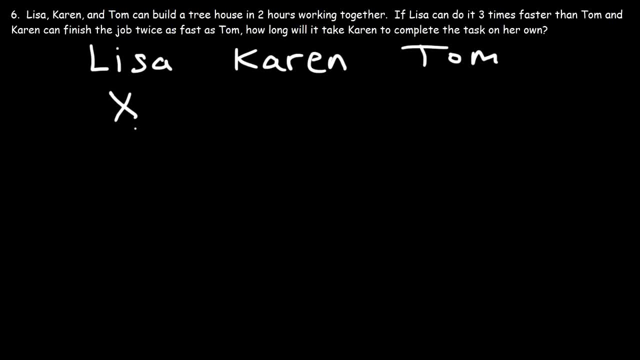 So if Lisa takes X hours, Tom is going to take three times X hours to get the job done. Now what about Karen? Karen can do the job twice as fast as Tom, which means Tom is twice as slow as Karen. So if Karen can do it in X hours, Tom can do it in two X hours or twice as long. 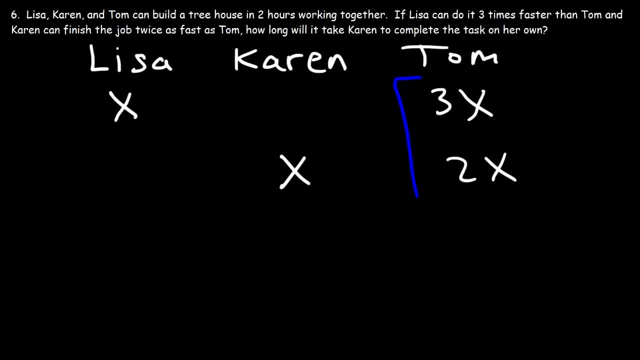 But now we can't have two different values. We can't have two different values for Tom, nor can we have the same value for Lisa and Karen. So how do we make this work? What do we need to do here? Hmm, Take a minute and try to figure it out. 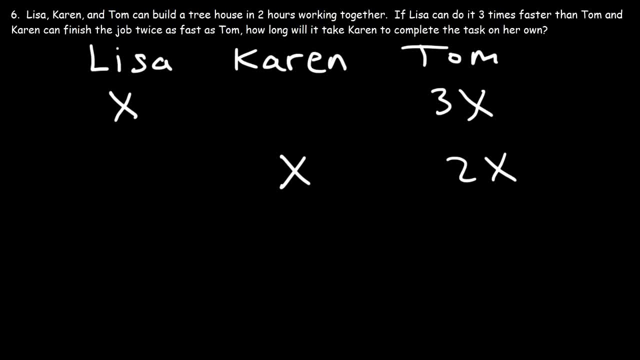 Pause the video and see if you can get the answer Now. somehow we need to make these two values the same. Now let's analyze this situation. If we divide both of those values by three, 3X divided by three will be X and X divided. 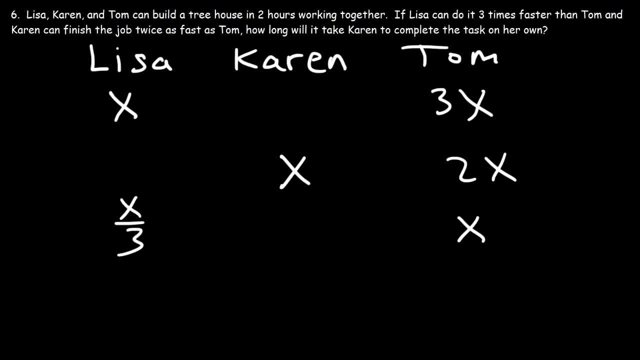 by three will be X over three. Now let's do the same for Tom and Karen, but we're going to divide it by two. 2X divided by two will give us X, And X divided by two is just 1.. So we're going to divide both of those values by three. 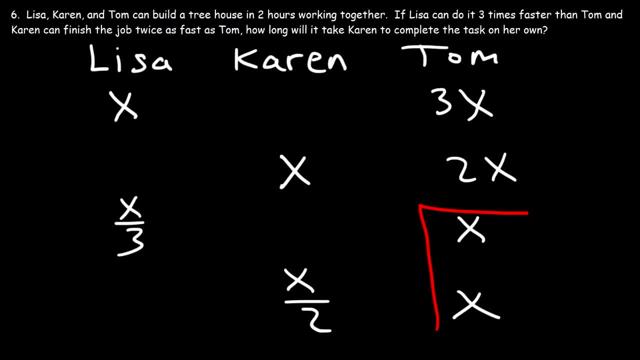 2X divided by two will give us X over two, And so now these two values are the same. So let's put this all together: If it takes Tom X hours to get the job done, then, Lisa, she could do it three times faster. 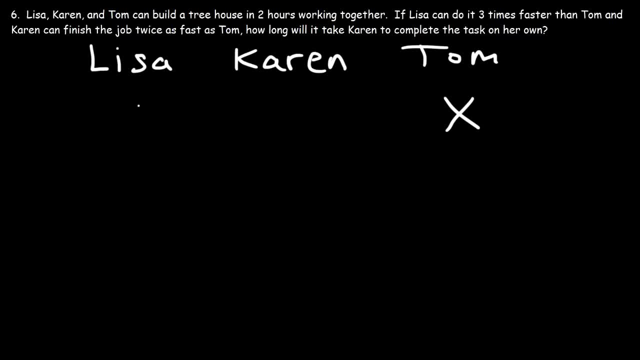 than Tom. So the time that it takes her will be whatever Tom's time divided by three. And Karen works twice as fast as Tom. So the time that it takes her will be whatever Tom's time divided by three, And Karen works twice as fast as Tom. 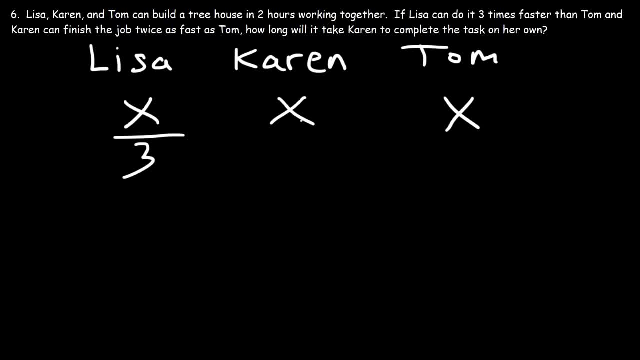 So, however long it takes Tom, it's going to take Karen half the time to get it done, because she works twice as fast as Tom, And so seeing it from this perspective makes it a lot easier, And now we can get the answer. 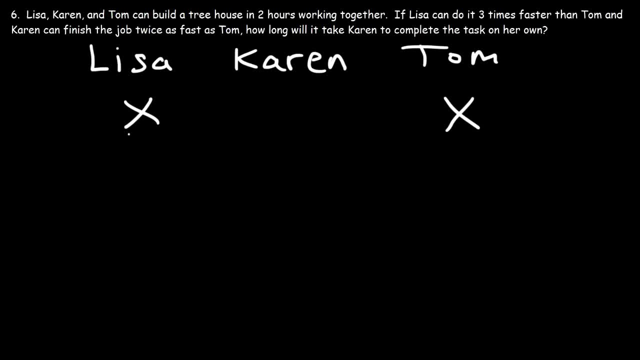 will be whatever Tom's time divided by three, And Karen works twice as fast as Tom. so however long it takes Tom, it's gonna take Karen half the time to get it done because she works twice as fast as Tom. And so, seeing it from this perspective, 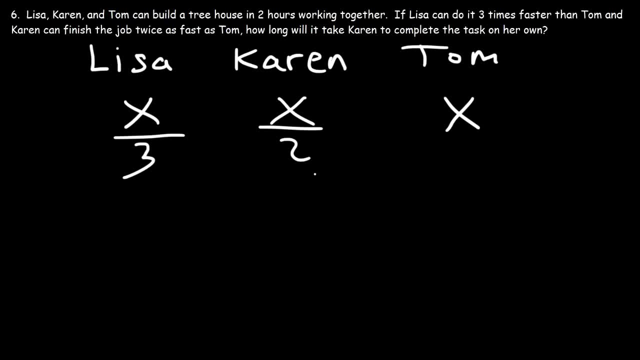 makes it a lot easier And now we can get the answer. So let's say that T sub L, K T again, that's the time it takes for Lisa, Karen and Tom to get it done, and that's going to equal 1 over TL plus 1 over TK, plus 1 over double T. now 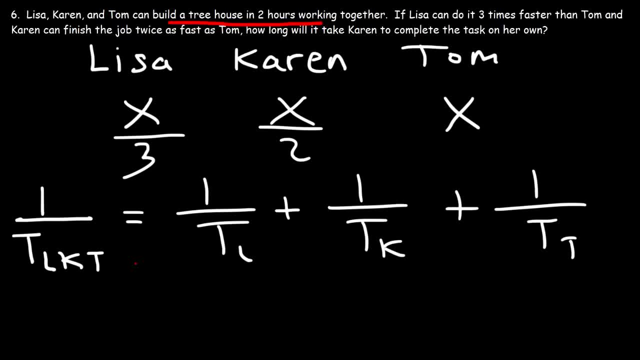 working together, they can build the tree house in two hours. so let's replace it, that value, with two. now the time that it's going to take Lisa to get it done. in terms of X, it's going to be X over 3, and for Karen it's X over 2, and for Tom it's. 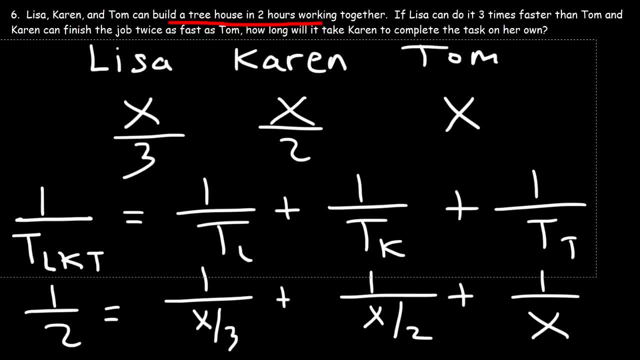 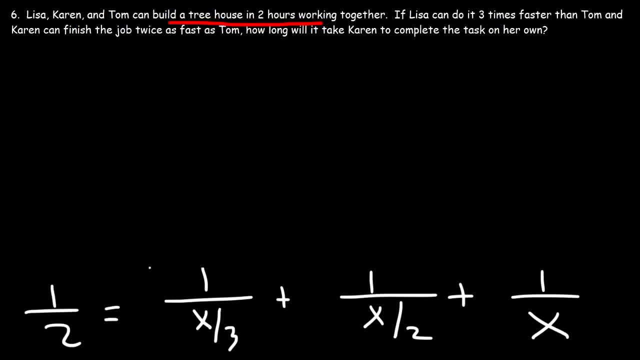 simply X. now let's simplify these fractions. what is 1 divided by X over 3? if we multiply the top and the bottom by 3- X over 3 times 3- those trees will cancel and so that becomes 3 over X. so you basically flip the fraction. so 1 over X over 2. just flip X over 2 and it's going. 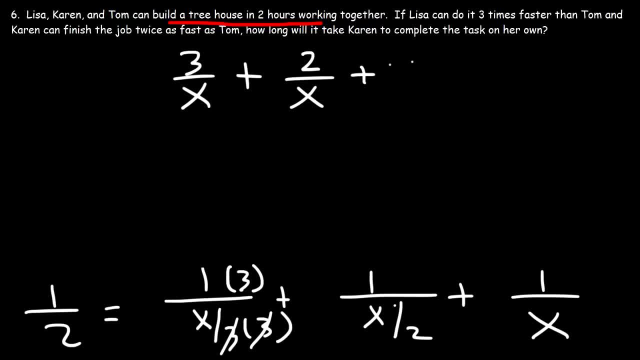 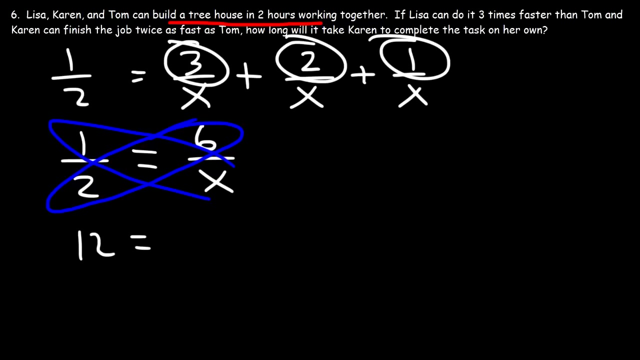 to become 2 of X, and so we have 3 plus 2 plus 1, which is 6. so we have: 1 over 2 is equal to 6 over X. now, at this point, what we need to do is cross multiply. so 2 times 6 is 12 and 1 times X is simply X. 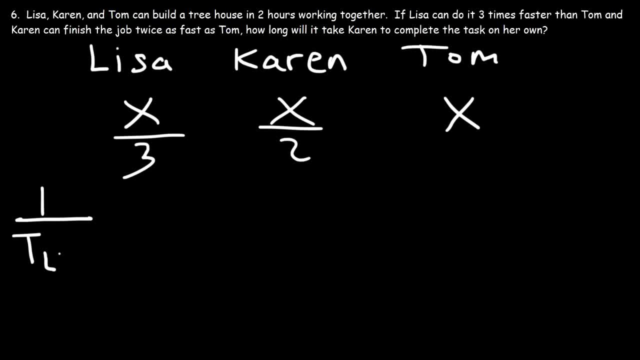 So let's say that T sub LKT again. that's the time it takes for Lisa, Karen and Tom to get it done, And that's going to equal one over TL plus one over TK plus one over TT. Now, working together, they can build the treehouse in two hours. 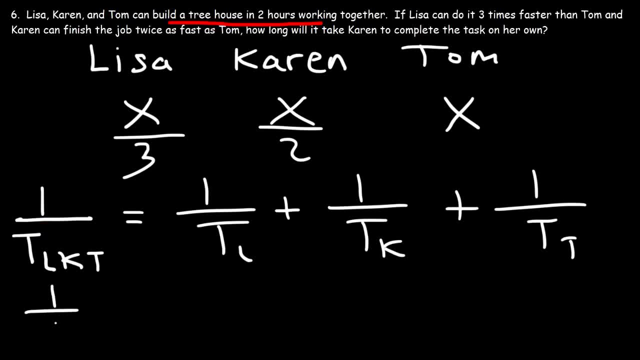 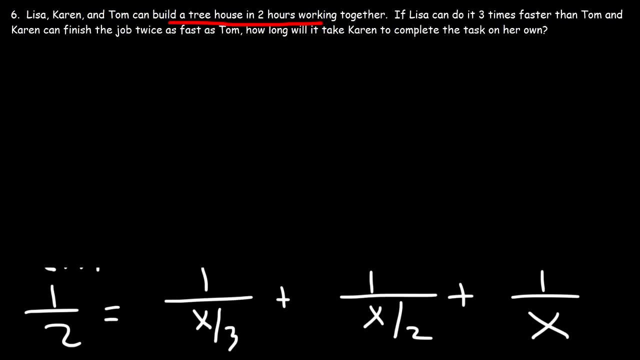 So let's replace that value with two. Now the time that it's going to take Lisa to get it done. in terms of X, it's going to be X over TK, And for Karen it's X over two, And for Tom it's simply X. 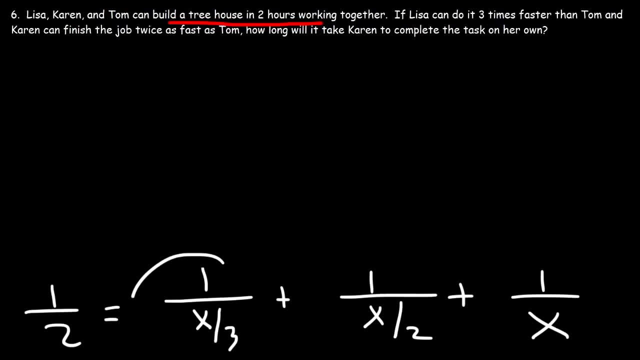 Now let's simplify these fractions. What is one divided by X over three? If we multiply the top and the bottom by three, X over three times three, those threes will cancel, And so that becomes three over X. So you basically flip the fraction. 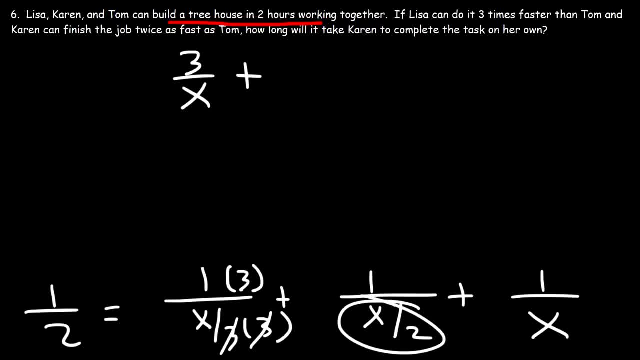 So one over X over two. just flip X over two and it's going to become two over X, And so we have three plus two plus one, which is six. So we have one over two is equal to six over X. Now, at this point what we need to do is cross multiply. 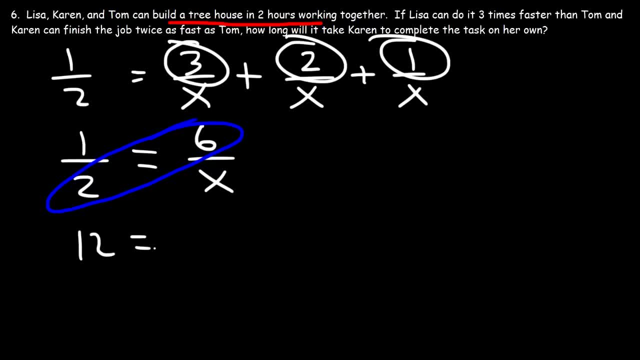 So two times six is twelve and one times X is simply X. So now we can finish the problem. So remember the time that it takes Tom to build it. we define it as X, which is twelve hours. The time that it takes Lisa to get it done, she works three times faster than Tom, so 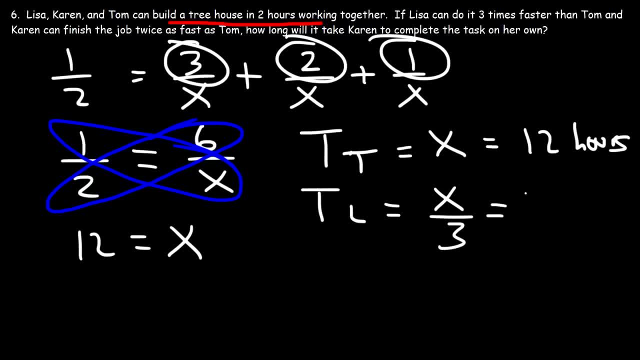 it's X divided by three, So twelve divided by three is four, And the one we're looking for is the time that it takes Karen to complete the task. Now she's working twice as fast as Tom, so she can get it done in half the time. 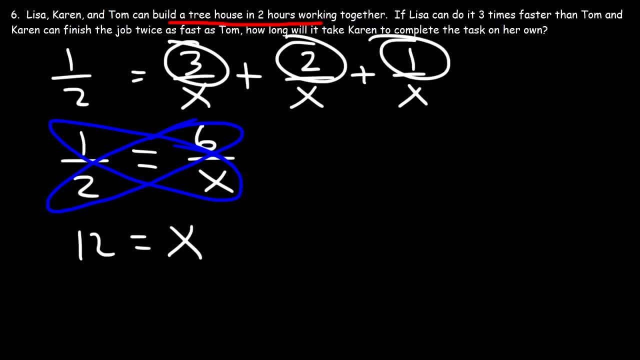 so now we can finish the problem. so remember the time that it takes Tom to build it. we define it as X, which is 12 hours, the time that it takes to Lisa to get it done. she works three times faster than Tom. so it's X divided by 3. so 12 divided by 3 is 4, and the one 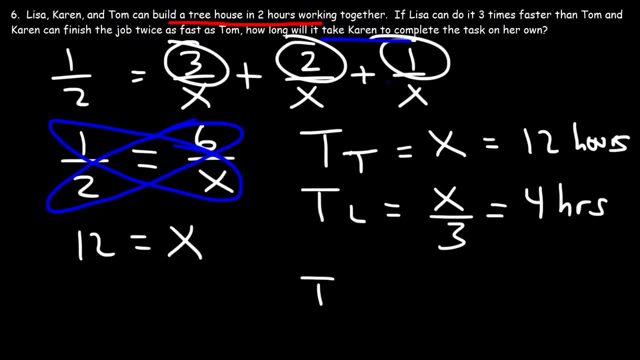 we're looking for is the time that it takes Karen to complete the task. now she's working twice as fast as Tom, so she can get it done in half the time. so 12 divided by 2 is 6 hours. therefore, this is the answer that we are looking. 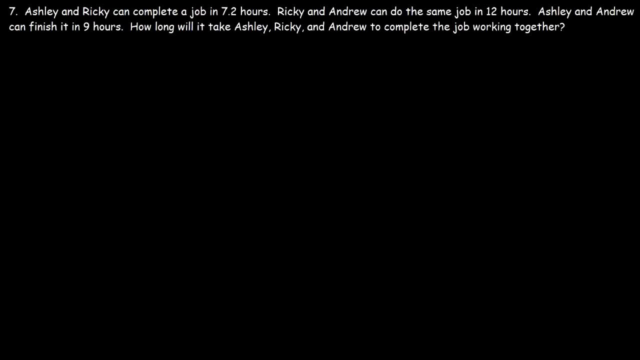 for 6 hours. so this is going to be the last question of this video. Ashley and Ricky can complete a job in 7.2 hours. Ricky and Andrew can do the same job in 12 hours. Ashley and Andrew can finish it in nine hours. how long will it take Ashley, Ricky? 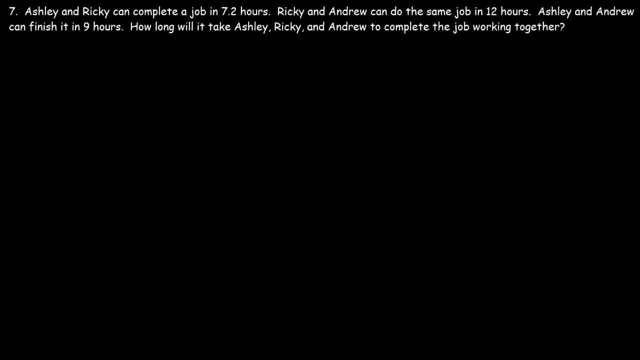 and Andrew to complete the job working together. so see if you can do this problem. take a minute and try it out. what do you think we need to do here? well, we know we could use this equation 1 over T, sub a for Ashley, our for Ricky. 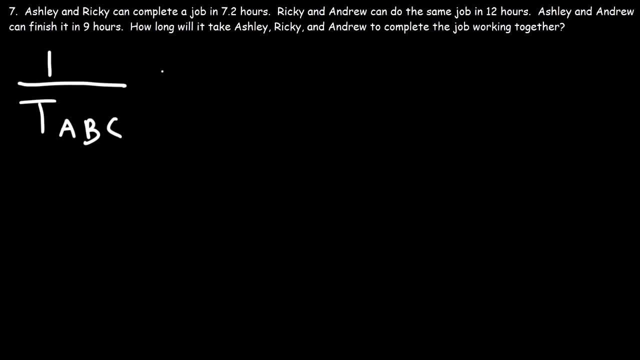 well, let's use a BNC B for Ricky and see for Andrew. that's going to equal 1 over ta plus 1 over TB plus one of the TC. however, the only problem is we don't have the time it takes for each individual to complete the task working alone. We don't have that. We. 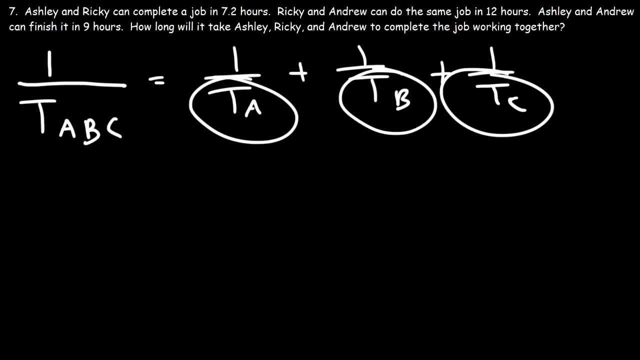 have the information for two individuals working together and we need to find how long it's going to take for all three individuals to get the job done. So we have the time for A and B. We also have the time for B and C and A and C. So how do we make this work? Well, we know that the time 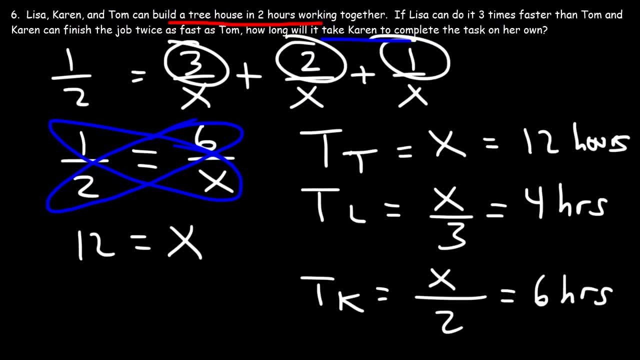 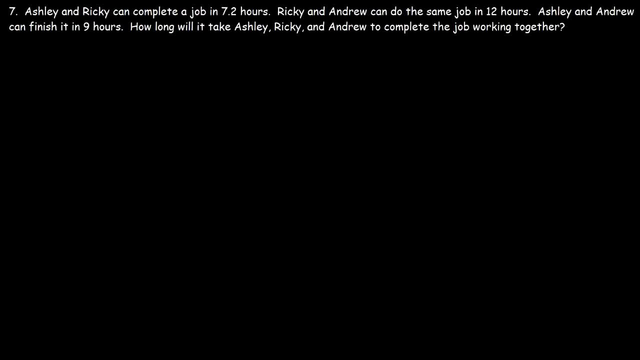 So twelve divided by two is six hours. Therefore, this is the answer that we are looking for: six hours. So this is going to be the last question of this video. Ashley and Ricky can complete a job in 7.2 hours. 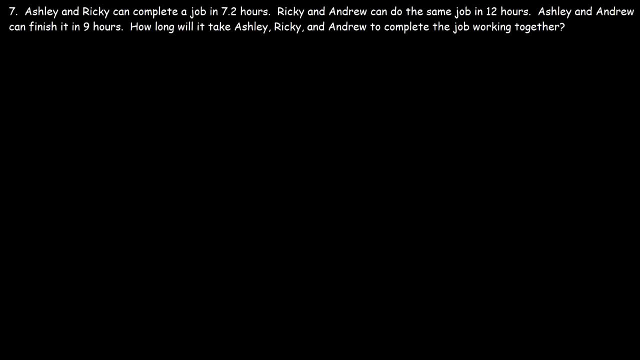 Ricky and Andrew can do the same job in 12 hours. Ashley and Andrew can finish the task in 12 hours, So this is going to be the last question of this video. Ashley and Ricky can complete a job in 12 hours, So this is going to be the last question of this video. 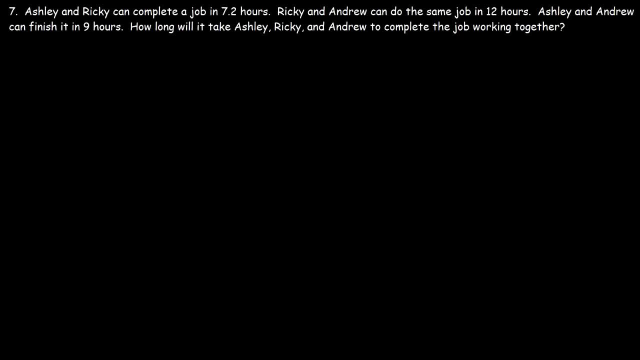 How long will it take Ashley, Ricky and Andrew to complete the job working together? So see if you can do this problem. Take a minute and try it out. What do you think we need to do here? Well, we know we could use this equation. 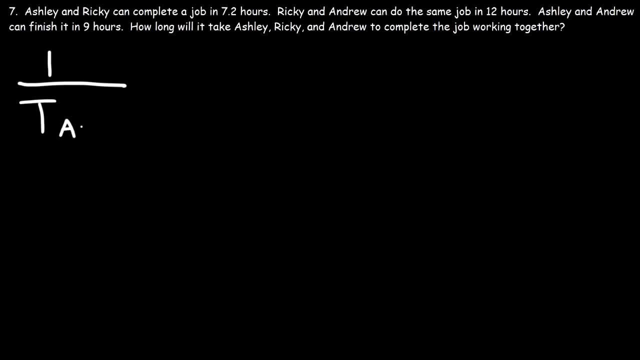 One over T, sub a for Ashley, Okay, R for Ricky. well, let's use A, B and C: B for Ricky and C for Andrew. That's going to equal 1 over T A, plus 1 over T B, plus 1 over T C. However, the only problem is we don't have 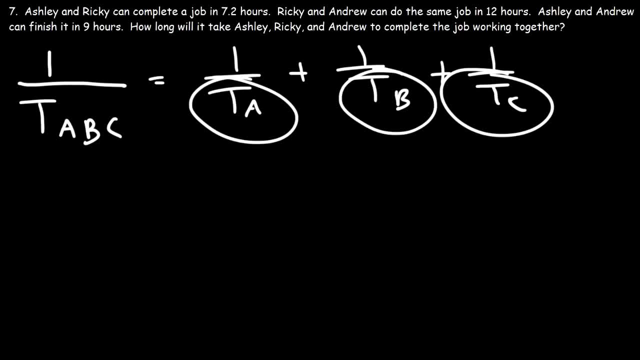 the time it takes for each individual to complete the task working alone. We don't have that. However, we have the information for two individuals working together and we need to find how long it's going to take for all three individuals to get the job done. So we have the time for. 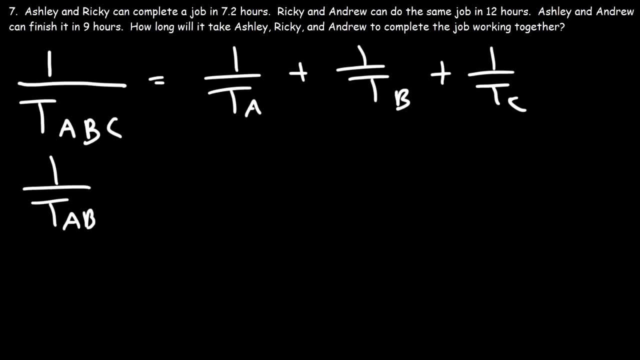 A and B. We also have the time for B and C and A and C. So how do we make this work? Well, we know that the time it takes for A and B to get it done is 1 over T, A plus 1. 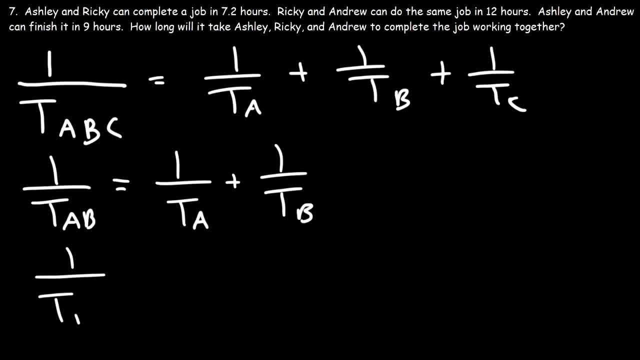 over T, C. So after we make that, we start to continue working. We also don't need to, And the time it takes for B and C- or let's say Ricky and Andrew- to get it done is 1 over TB plus 1 over TC. 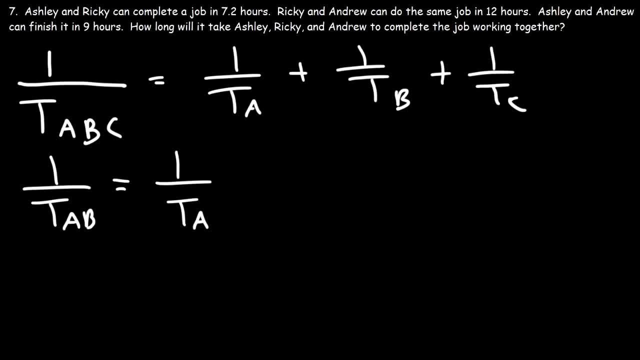 it takes for A and B to get it done is 1 over t A plus 1 over t B, And the time it takes for B and C, or let's say Riki and Andrew, to get it done is 1 over t B plus 1 over t C And the 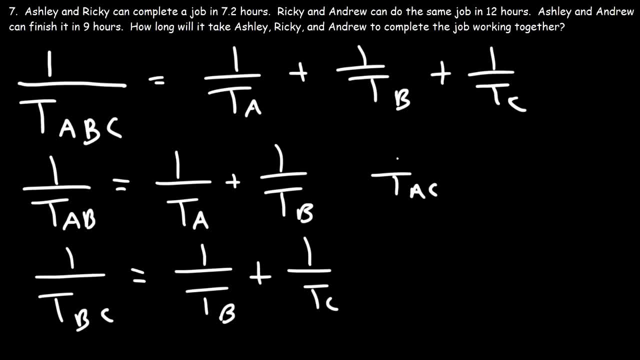 time it takes for Ashley and Andrew to get it done is going to be a little more than one hour. て doing is going to b 1 over ta plus 1 over TC. so how do we combine all of these equations and make them work? so, basically, how do we find the time it takes for a BNC working? 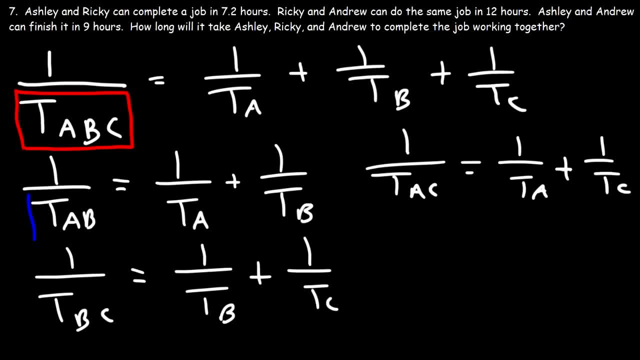 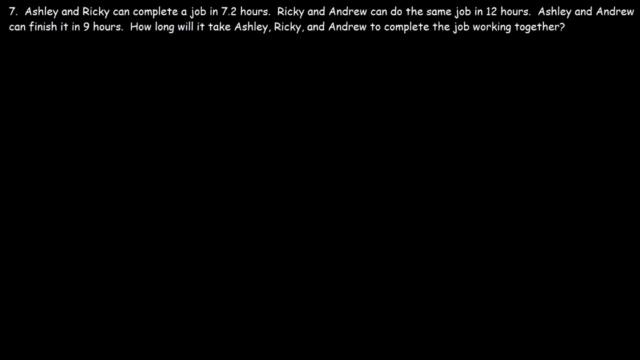 together using the time of a and B, working together BNC and ANC. if we can write an equation that has these four variables in it, then we can get the answer. so let's start with this expression: 1 over T a B plus 1 over T, BC. 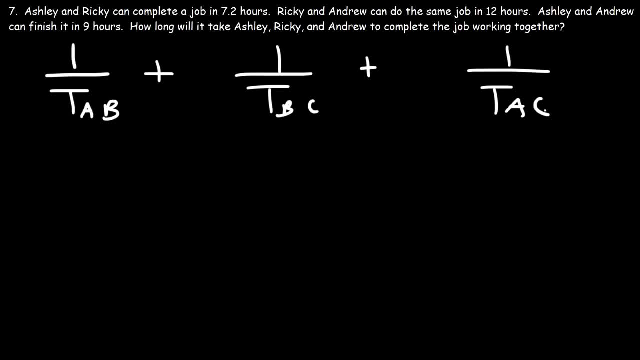 plus 1 over T a C. keep in mind: a is for Ashley, B is for Ricky and C is for Andrew. so let's replace that expression with 1 over T a plus 1 over TB, now 1 over T BC. that's going to be 1 over TB plus 1 over TC and 1 over T a C. 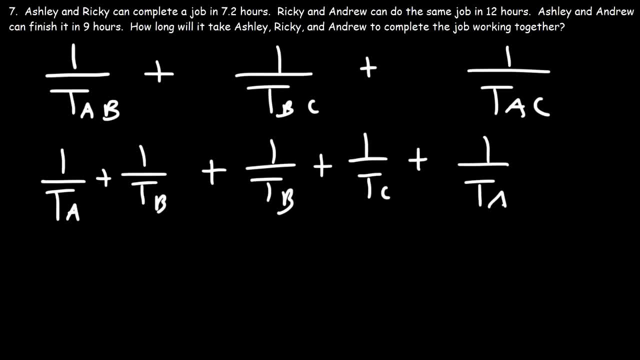 as we wrote previously, it's one of a TA plus 1 over TC. now let's put an equal sign. so this expression here is equal to everything that we see below it. now let's combine like terms, so 1 over T a plus another 1 over T a. we could say that's 2 over T a. let me conserve space. 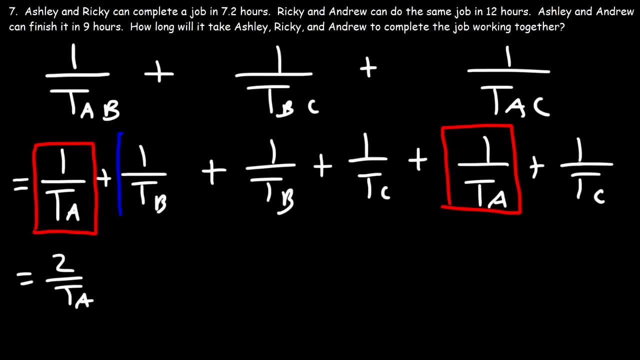 and then we could do the same away from 1 over TB. if we add that, I mean, excuse me, if we add those two, it's going to be 2 over TB, and the same is true for the last two variables. so that's going to be 2 over TC if we 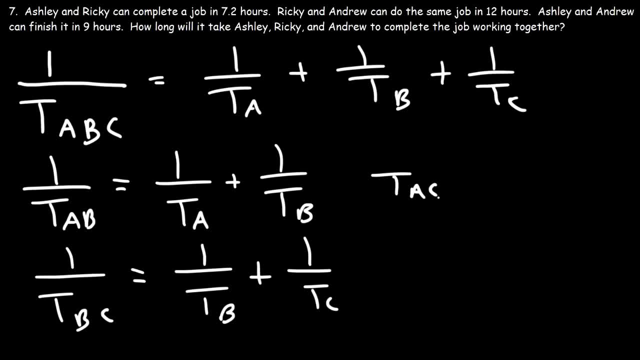 And the time it takes for Ashley and Andrew to get it done is going to be 1 over TA plus 1 over TC. So how do we combine all of these equations and make them work? So, basically, how do we find the time it takes for A, B and C working together, using the time of A and B working together, B and C and A and C? 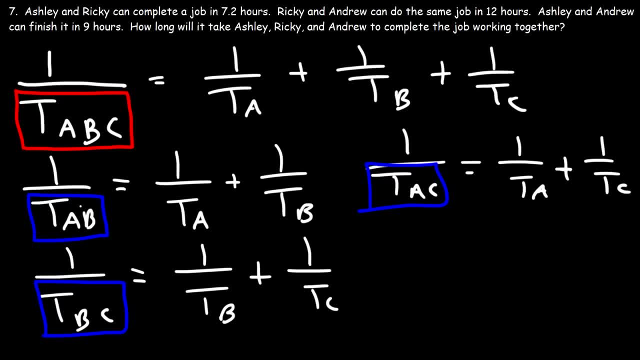 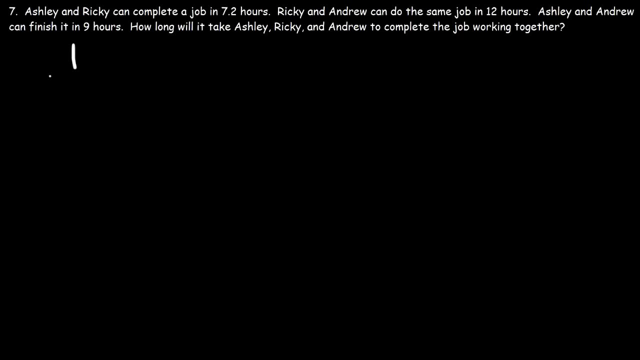 If we can write an equation that has these four variables in it, then we can get the answer. So let's start with this expression: 1 over TAB plus 1 over TBC plus 1 over TAC. Keep in mind: A is for Ashley, B is for Ricky, C is for Andrew. 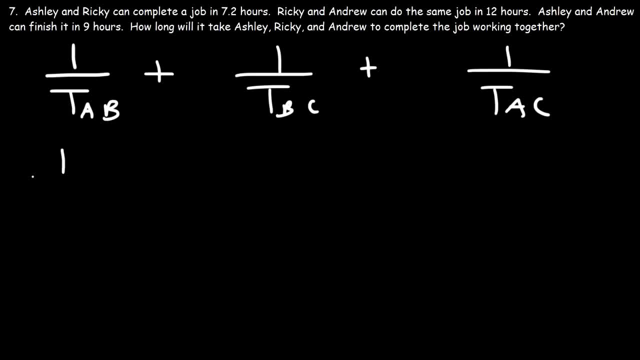 So let's replace that expression with 1 over TA plus 1 over TB, Now 1 over TBC. that's going to be 1 over TB plus 1 over TC And 1 over TAC. as we wrote previously, it's 1 over TA plus 1 over TC. 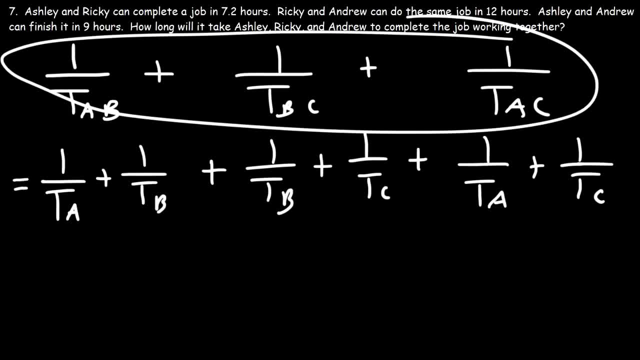 Now let's put an equal sign. So this expression here is equal to everything that we see below it. Now let's combine, Now I like terms, So 1 over TA plus another 1 over TA, we could say that's 2 over TA. 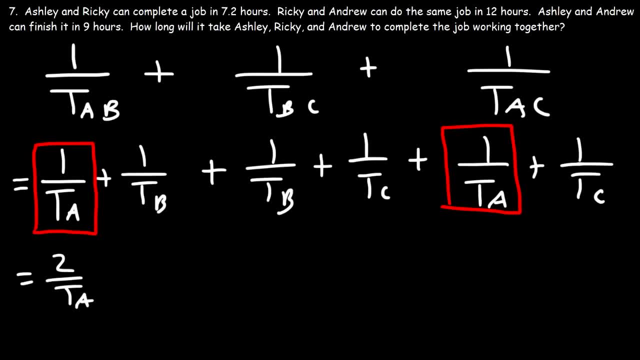 Let me conserve space. And then we could do the same with 1 over TB. If we add that, I mean, excuse me, if we add those two, it's going to be 2 over TB. And the same is true for the last two variables. 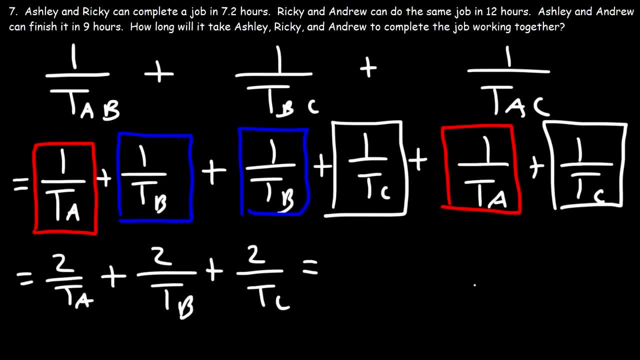 So that's going to be 2.. If we factor out the two, this is going to equal 2 times 1 over TA, plus 1 over TB plus 1 over TC. Now this here is equal to simply 1 over TABC. 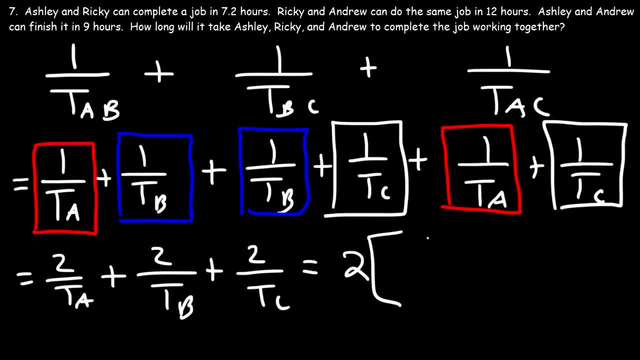 factor out the 2, this is going to equal 2 times 1 over T a, plus 1 over TB, plus 1 over TC. now this here is equal to simply 1 over T a BC. so that's the time that it takes for a, B and C working. 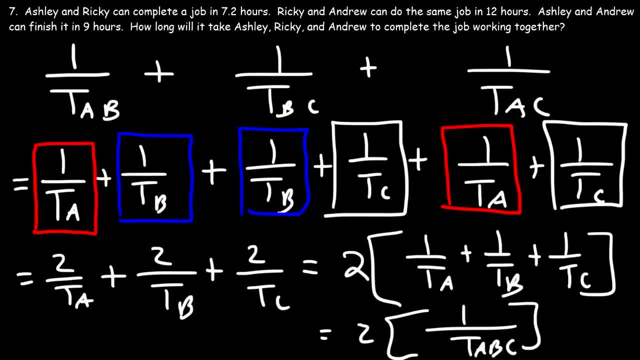 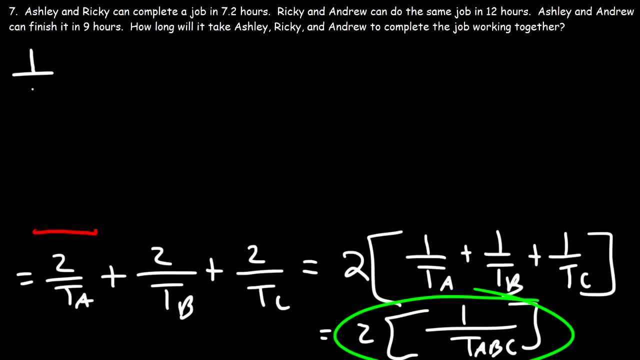 together so understand that this expression is equal to what we see here. so we could say that 1 over T a B plus 1 over T BC, plus 1 over T a C, all of that is going to equal 2 times 1 over T a BC. so that's the formula that we need for this problem. now, T a B, that's. 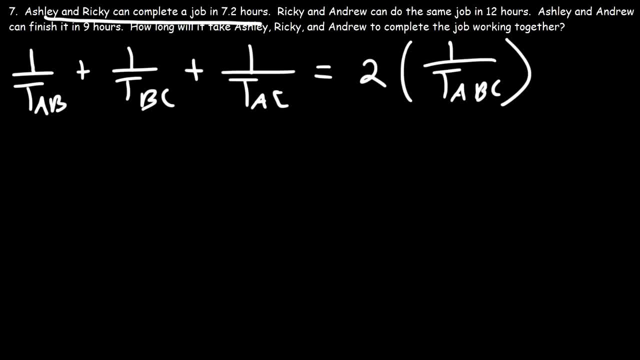 the time it takes for Ashley and Ricky to complete the job, which is 1 over T a B, and Ricky to complete the job, which is 7.2 hours T BC. that's the time it takes for Rick and Andrew to complete that same job, which is 12 hours, and T a C is. 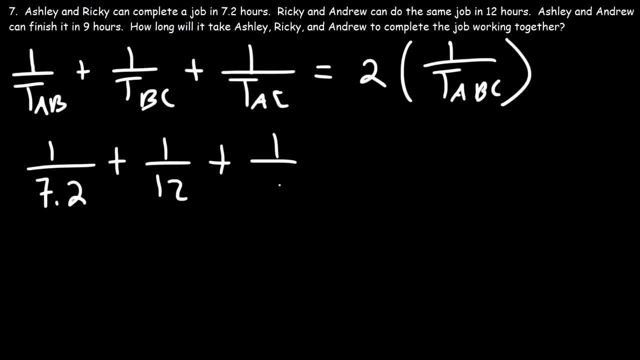 for Ashley and Andrew, and they could do it in 9 hours. now we're looking for this- the time that it takes for all of them to get the job done, and so let's replace T, A, B, C with X. So our goal is simply to calculate X. Now how can we do this? 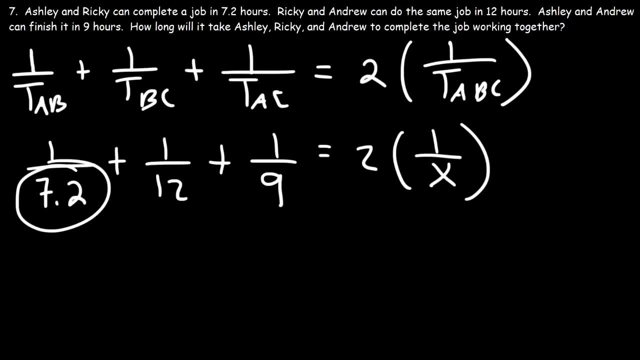 since we have a decimal number. So how can we find the LCM of 7.2,, 12,, 9, and X? Well, let's focus on the 0.2.. 0.2 times. what number will give us a whole number? 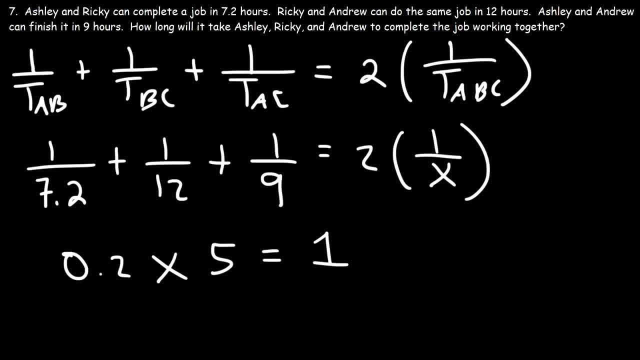 It turns out that 0.2 times 5 is 1,, just as 2 times 5 is 10.. Now what is 7.2 times 5?? 7 times 5 is 35.. 0.2 times 5 is 1.. If you add 35 and 1,, you get 36.. So 7.2 times 5 is 36.. 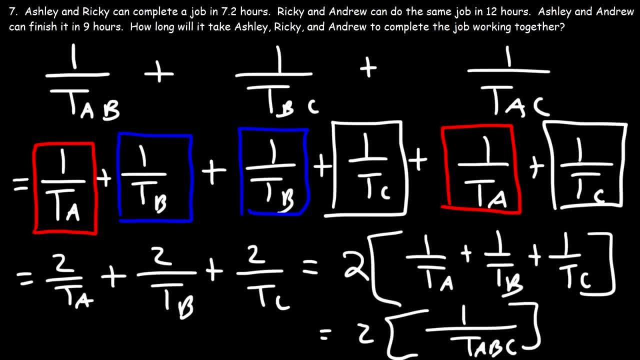 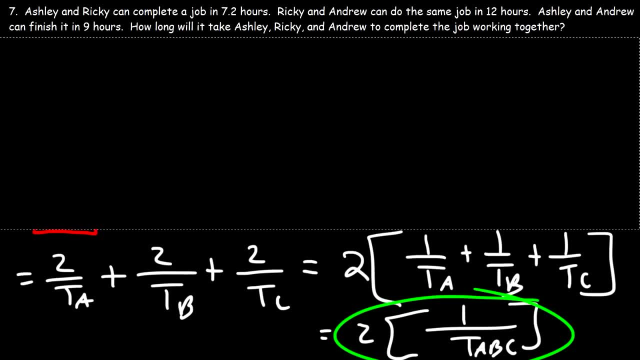 So that's the time that it takes for A, B and C working together. So understand that this expression is equal to what we see here. So we could say that 1 over TAB, plus 1 over TBC, plus 1 over TAC. 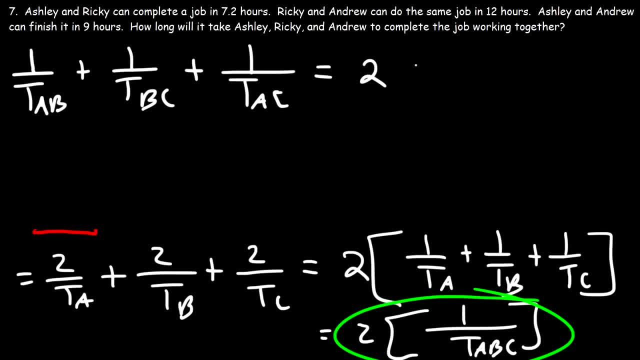 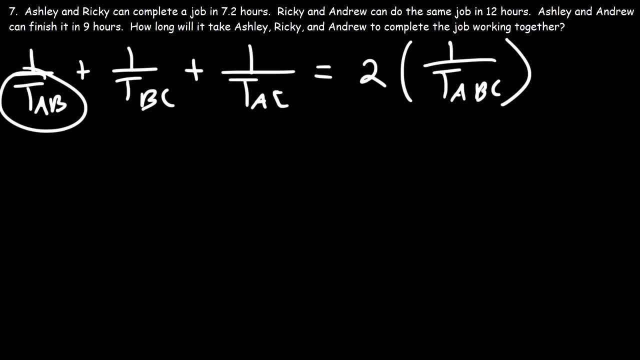 All of that is going to equal 2 times 1 over TABC. So that's the formula that we need for this problem. Now, TAB: that's the time it takes for Ashley and Ricky to complete the job, which is 7.2 hours. 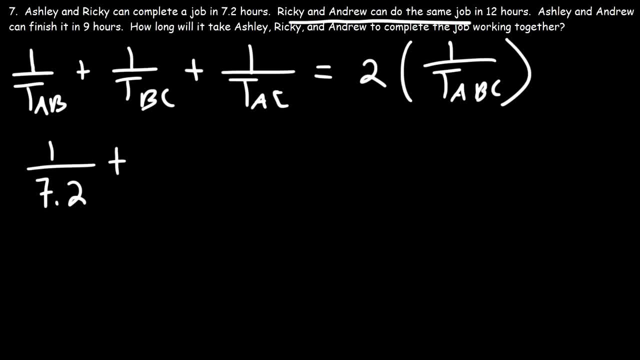 TBC. that's the time it takes for Ricky and Andrew to complete that same job, which is 12 hours, And TAC is for Ashley and Andrew, and they could do it in 9 hours. Now we're looking for this- the time that it takes for all of them to get the job done. 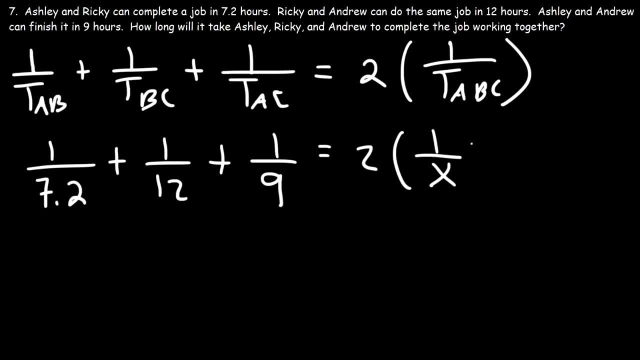 And so let's replace TABC with X. So our goal is simply to calculate X. Now, how can we do this, since we have a decimal number? So how can we find the LCM of 7.2,, 12,, 9, and X? 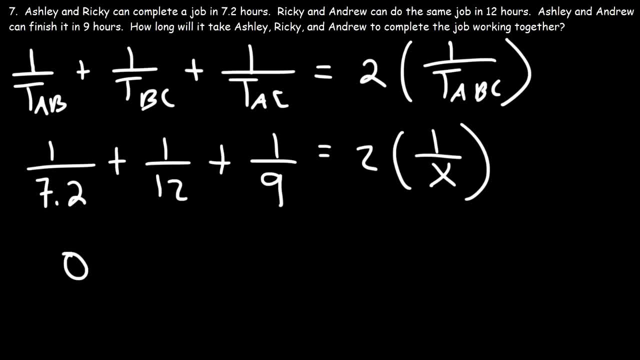 Well, let's focus on the .2.. .2 times what number will give us a whole number? It turns out that .2 times 5 is 1,, just as 2 times 5 is 10.. Now, what is 7.2 times 5?? 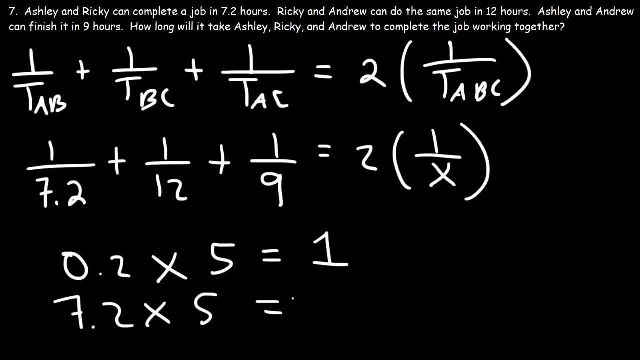 7 times 5 is 35.. .2 times 5 is 1.. And if you add 35 and 1, you get 36.. So 7.2 times 5 is 36.. And it turns out that 9 and 12, they both go into 36..